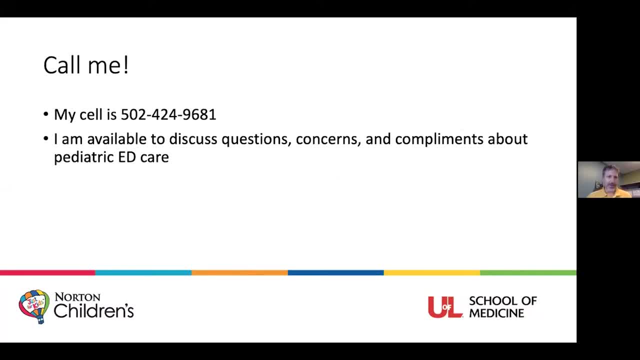 That's my cell phone number right there. Why don't you copy it down? or, if you want, go ahead and send me a text right now and introduce yourself. We operate three emergency departments here in the city and I would really like the opportunity to hear from you. 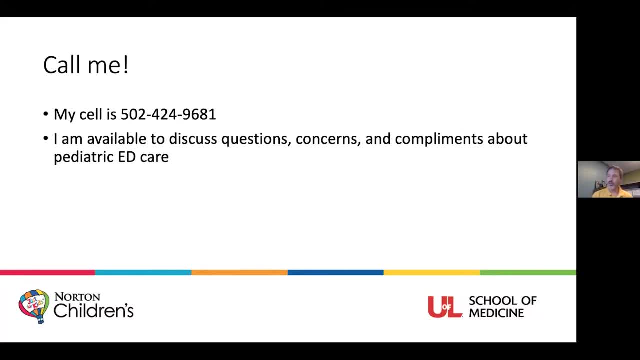 you and talk to you about any questions or concerns or things we can do to enhance pediatric ED care for your patients. So please feel free to somebody just did reach out to me. feel free to reach out to me and talk to me whenever you want. I'll ask McKenna to put that number in the chat. 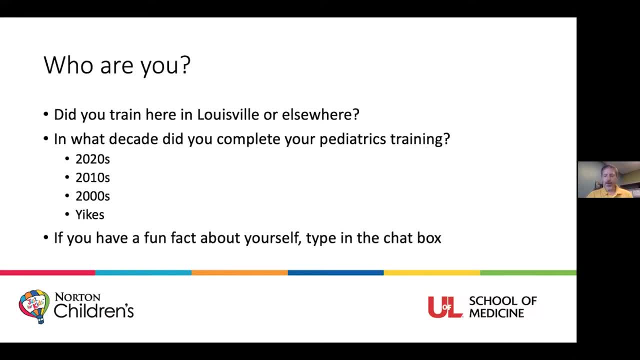 in case you didn't copy it down, All right, so there's a couple of poll questions that I asked McKenna to help me with here, just to keep this interesting. So I want to know where you trained first of all, if you trained here or if you trained somewhere else. 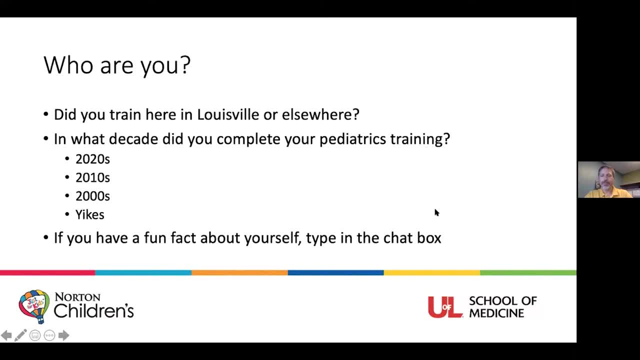 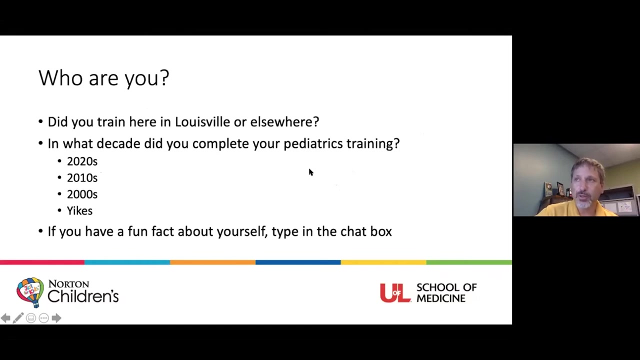 Looks like I have to answer it too, So I'll give that a moment. All right, so it looks like: wow, 50-50,. really right on the nose, That's pretty impressive. Okay, so half of people trained here in Louisville and are perhaps familiar with you know how things. 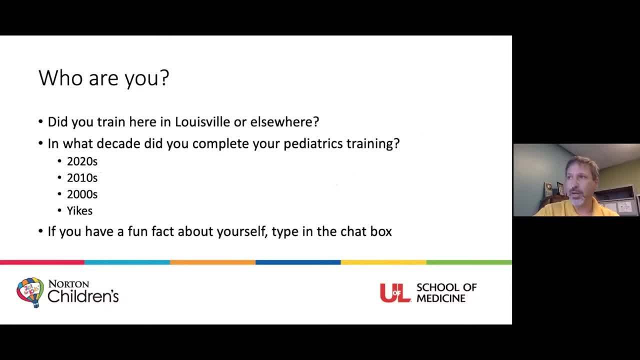 have been done here traditionally in the city, and others you know have formed their views of how things are done based on training elsewhere. So the next question is: what decade did you complete your pediatrics training? I'll give that a moment. Hope everyone's paying attention. 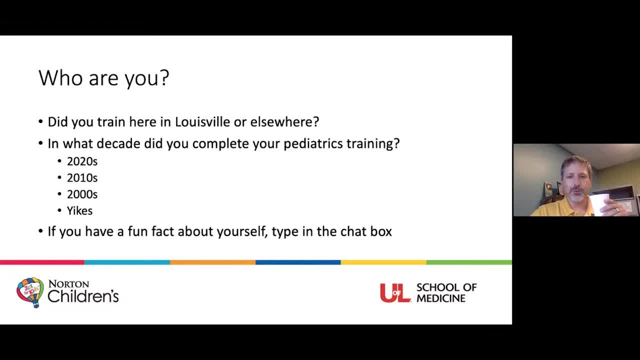 All right. so it looks like quite a few of you trained, you know, let's say, more than 10, 20 years ago, And I think this talk will be especially relevant because we're really going to talk about some things that have changed just in the last few years in how we manage some of 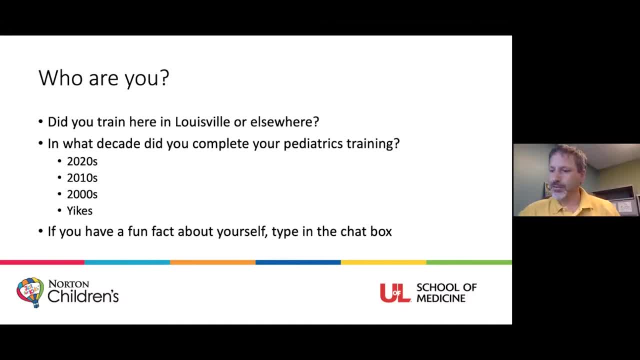 these conditions. And then this last one: you know, if you have a fun fact- and I already sort of gave you mine- go ahead and put it in the chat box- although I actually can't see the chat box so I can't monitor that- But go ahead. I guess you all can look at them. 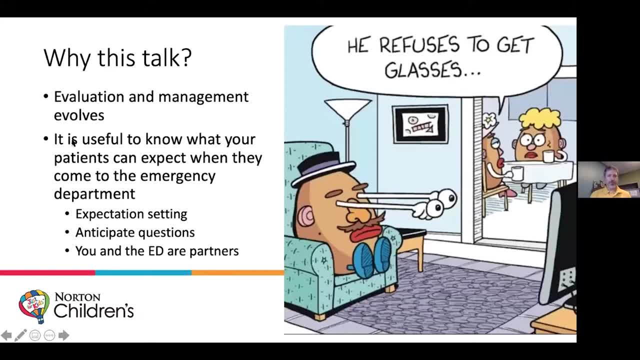 All right. so again, why are we doing this? Really? the reason is because evaluation and management of pediatric patients- all patients evolves and it's useful to know, for you, to know, what your patients can expect when they come to our emergency department. You can help us with. 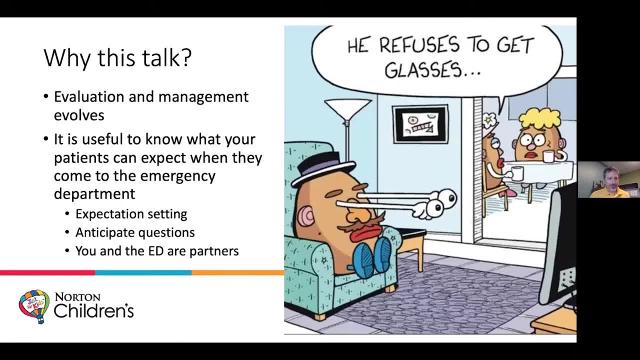 setting expectations. you can anticipate, maybe, questions that they have and understand the answers, And really we're in partnership with you on this. So if you understand what our current management is, it's really going to help you and us take better care of your patient. 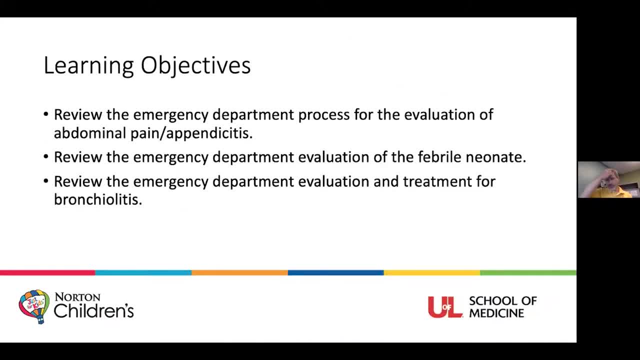 So these are the learning objectives for this talk. You can see them there quickly And these were already provided to you. But we're going to basically talk about abdominal pain, febrile neonates and bronchiolitis. But I actually changed the order of how I did this, And the reason is: 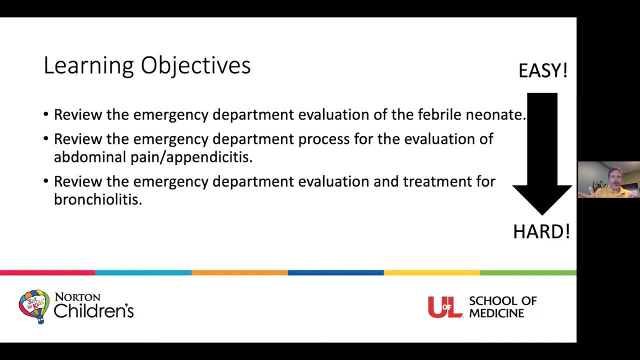 I think the evaluation is much more straightforward and clear cut for a febrile neonate than it is for bronchiolitis, for example, with abdominal pain sitting somewhere in the middle. And the reason for that is that you know, the febrile neonate is objective and we have a bunch of objective. 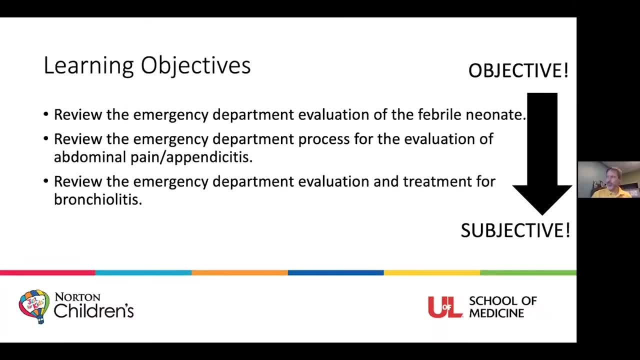 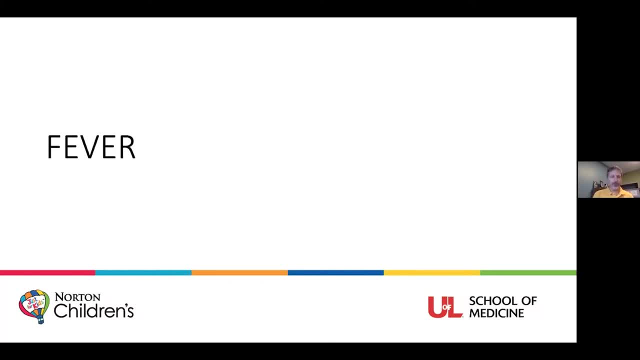 findings: mostly the fever, whereas bronchiolitis has a lot more subjective component to it, And so I've changed the way we're going to talk about this. So I want to start off easy, And that's with fever, And again we're talking about febrile neonates. 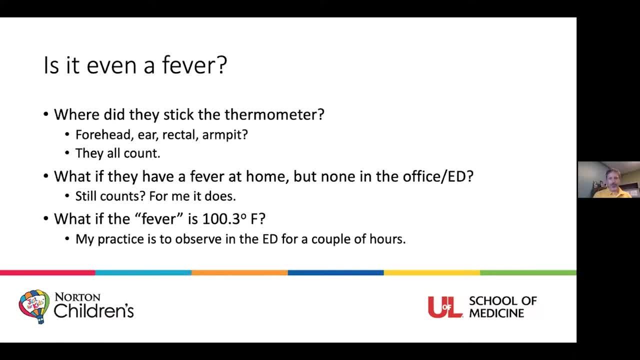 You know, and one of the questions that we sometimes have to answer is: is it even a fever? And I think you folks know this. but you know where the thermometer goes is somewhat important. You know, frankly, if somebody reports to me that they did a forehead or an ear temperature and they had a, 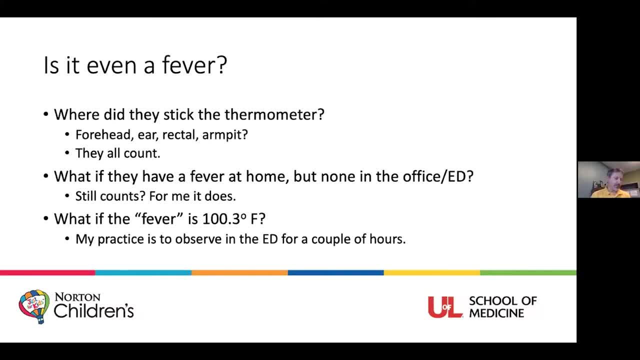 temperature of 101 or 100.4 or greater. I'm going to evaluate that just as I would a rectal temperature. Again. if they have a fever at home, but they come to your office and then they show up in my emergency department and they don't have a fever, what do I do with that? Well, for me, 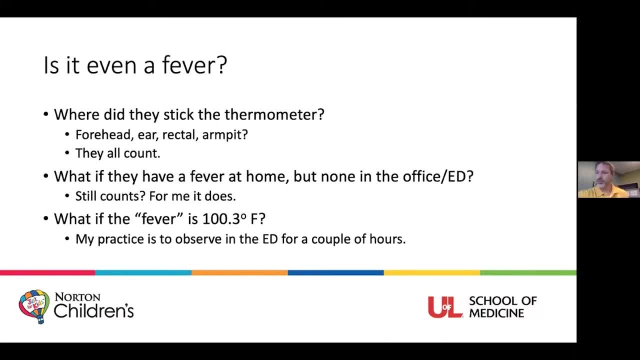 in the way all of the literature has been done in the past, that still counts, so to speak, as a fever. And then what if the fever is 100.3? You know what do we tend to do with that, And for the most part we're just going to observe those. 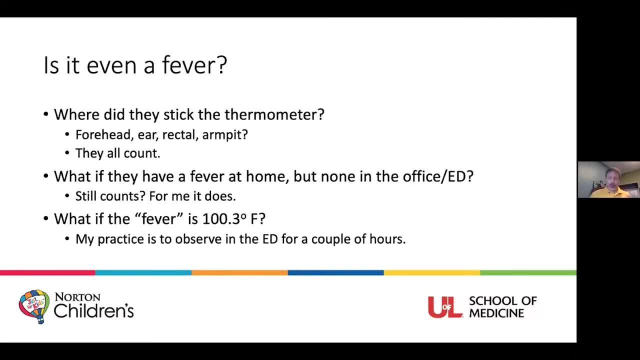 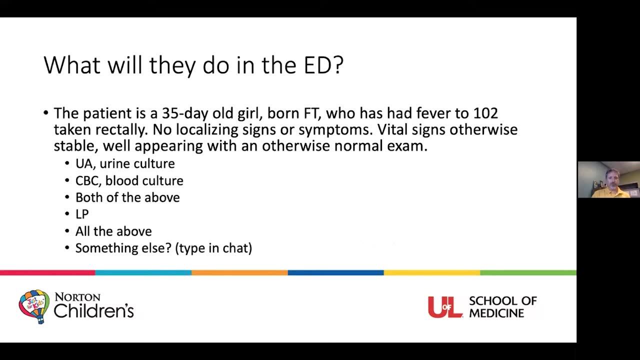 kids, Make sure they look well, check vital signs for a couple of hours serially, including temperatures, And if after two or three hours they're still a febrile without any antipyretics, we will usually let them go. That's not really what this talk is about, So let's let me propose: 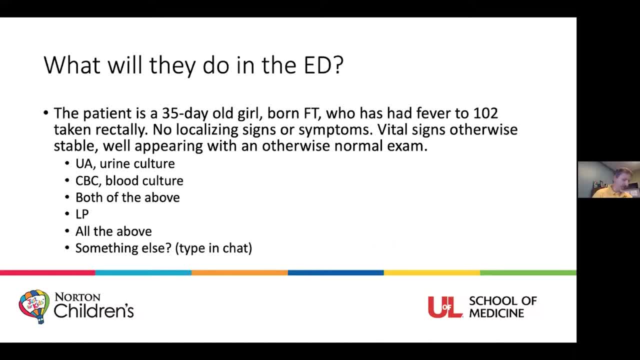 a case to you And again you're going to have to, you're going to have to answer a question. So you have a 35 day old girl who was born full term, who had had a fever to 102 taken rectally. Suppose this was in your office, it was 102.. 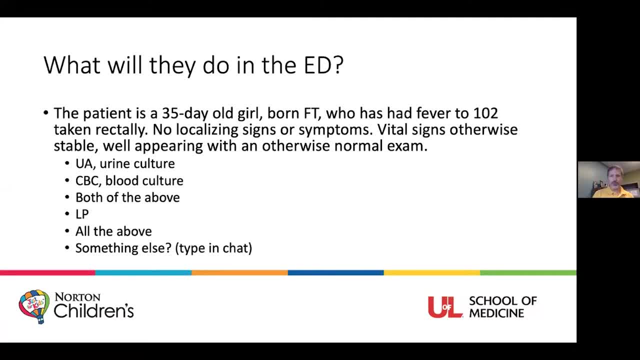 No localizing signs or symptoms. vital signs were stable and she's well appearing with a normal exam. So you say, well, you need to go to the emergency department, you're a baby, a neonate, with a fever. What will they do in the emergency department? What will we do in the emergency? 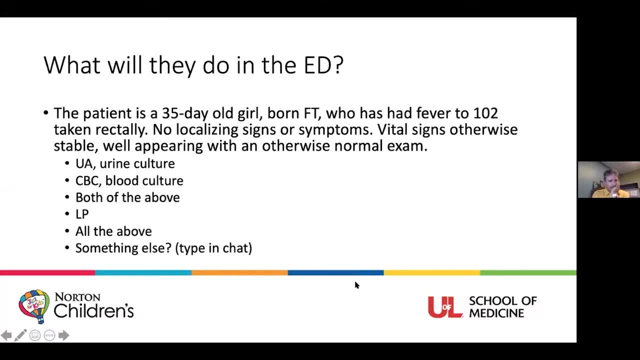 department. I'm going to give you a moment here to consider. I cannot see the chat, actually, All right, So looks like we're pretty 50- 50 on this 35 day old girl. So let's see, So let's see. 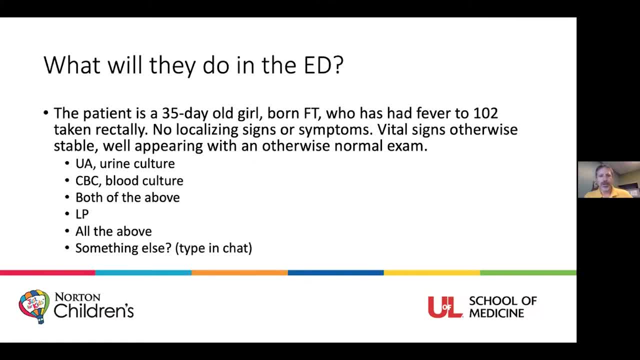 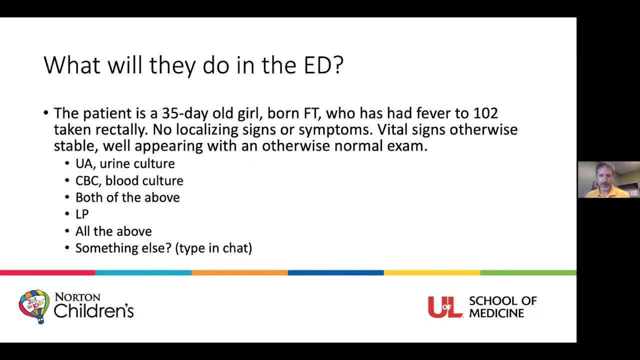 half of you saying we're going to do those things plus a lumbar puncture. So, and again, I don't know if anybody put anything interesting in the chat, but let's just go with that, because that's kind of what I wanted you to say And I. we probably should have seen how it's split out. 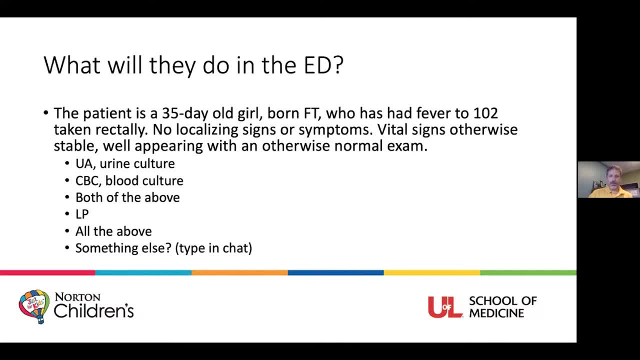 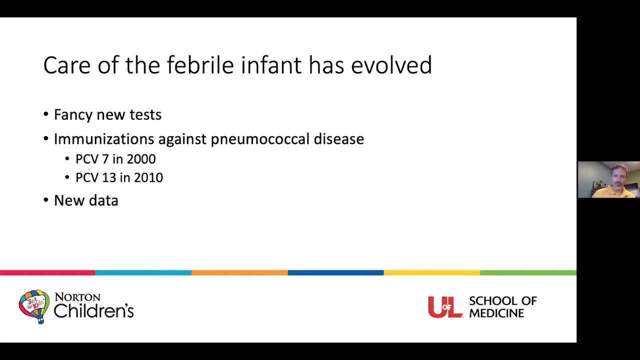 based on when you train. that might've been interesting, But you know, the care of these febrile neonates has evolved. There's new testing that we do, There's immunization now against pneumococcal disease and there's new data that's come out, even just in the last couple of years. 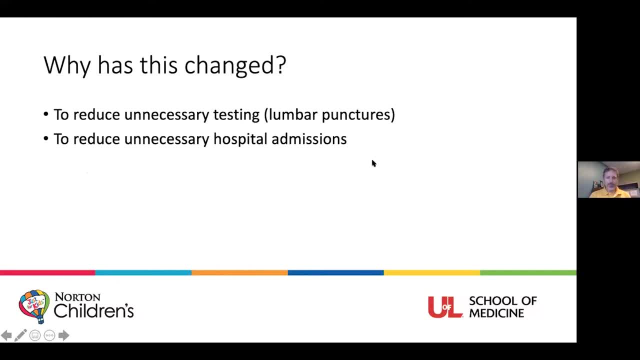 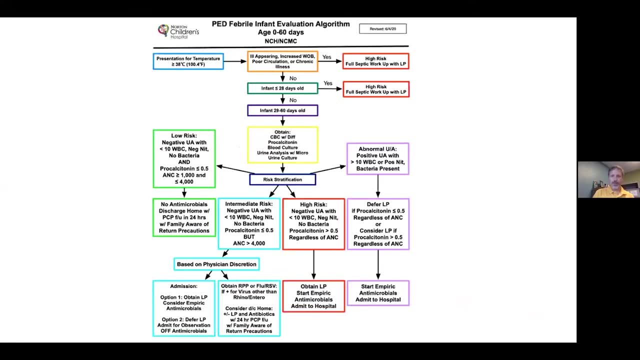 And why has our practice evolved? Well, we want to reduce unnecessary, unnecessary testing, We want to reduce unnecessary hospital admissions, And so this is an algorithm, and I'm going to focus in on different parts of this, So you don't need to take the whole thing in all at once. You will note that this algorithm was just revised, in June. 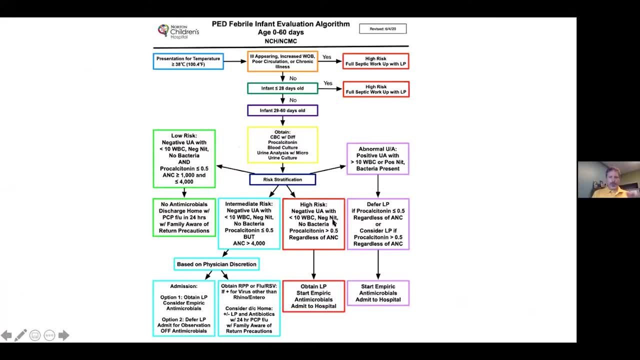 of last year. right, So it was. it was an algorithm that was designed to reduce unnecessary hospital admissions, And so this is an algorithm that was designed to reduce unnecessary hospital admissions right in the middle of the pandemic. We're going to slowly focus in on parts of this. I'm going to 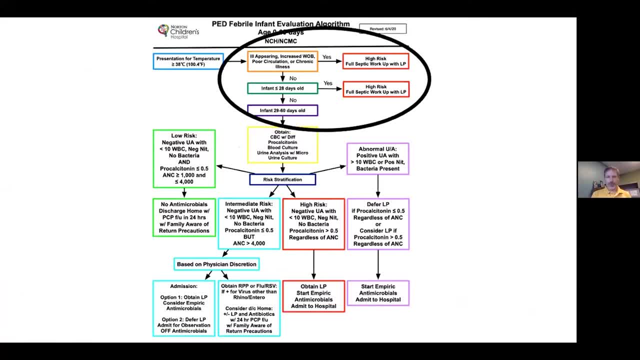 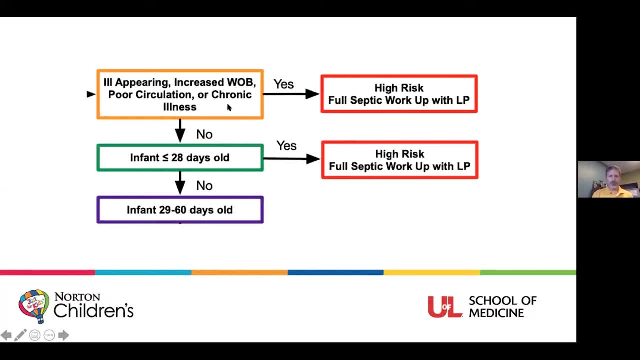 walk you through what we do and why. So we're going to start up here, I'm going to blow this up, So that first box that's in that yellow orangey color, this one, if you can see my pointer. So if a child is ill appearing or not breathing well, or doesn't have good circulation or has 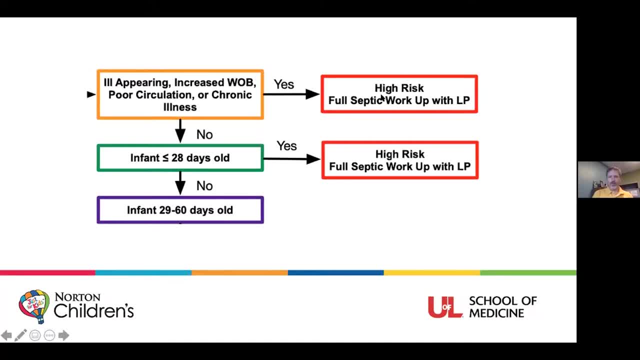 some chronic illness. no matter what, they're considered high risk and they get the blood, urine and lumbar puncture. Moreover, if a child is less than 28 days old with a fever, they're also high risk and we'll get that full evaluation. It is in this purple box. 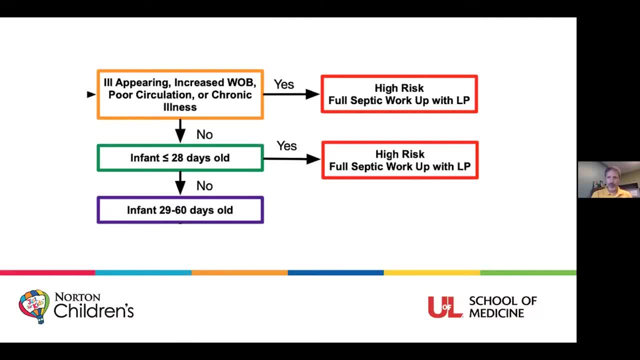 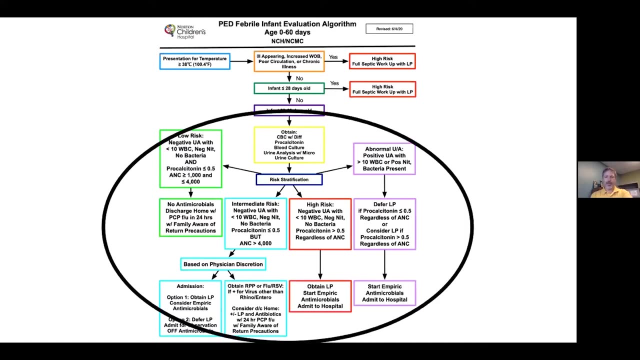 the children who are 29 to 60 days old. that's where things have changed And, again, this was June of last year that we formally adopted this algorithm. So back to the whole algorithm. Now we're going to walk back through sort of what happens in these children who are 28 to 60 days. 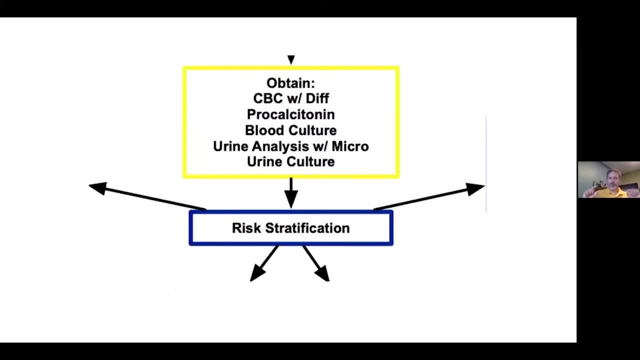 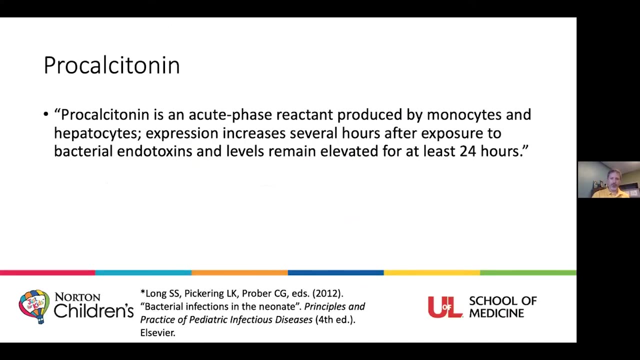 old, All right. So we're going to start with CBC, blood culture, UA and urine culture, and then this thing in the middle, procalcitonin, which has been around for a while in various instances. And just to review, procalcitonin is an acute phase reactant that's produced by monocytes and 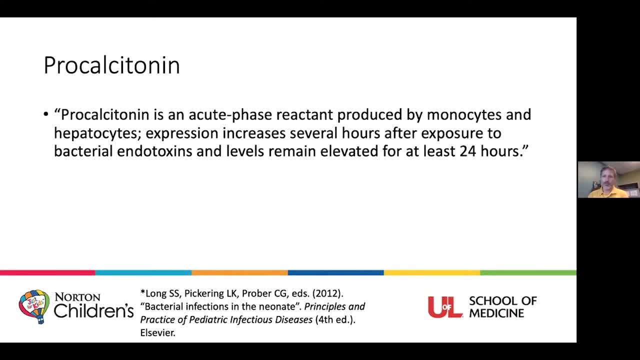 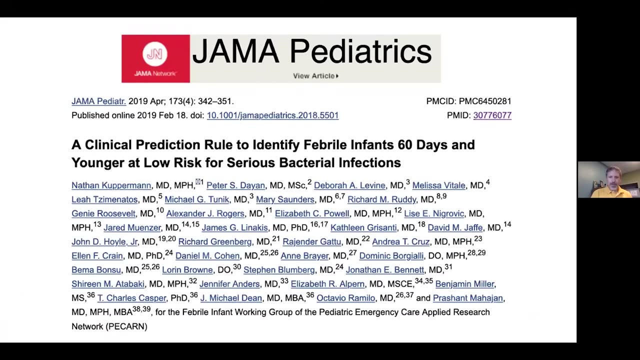 hepatocytes Expression increases several hours after exposure to bacterial endotoxins, and levels remain elevated for at least 24 hours, And so this has been looked at as a marker for bacteremia and sepsis, And that's why it's important, And so it was so important, And you can see this article. 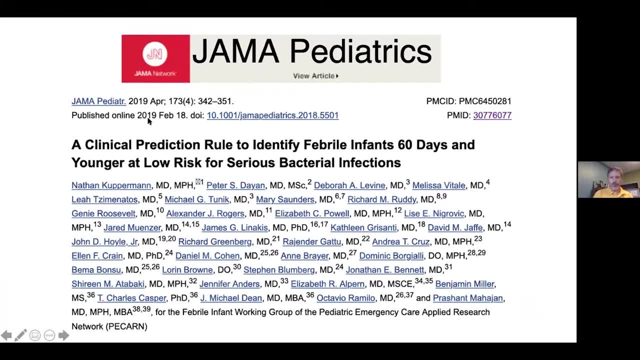 was in JAMApedes in February of 2019.. And this data was published through this pediatric emergency care applied research network, what we call PCARN. This is a NIH funded national consortium of pediatric emergency departments, And so they did a prospective trial looking at 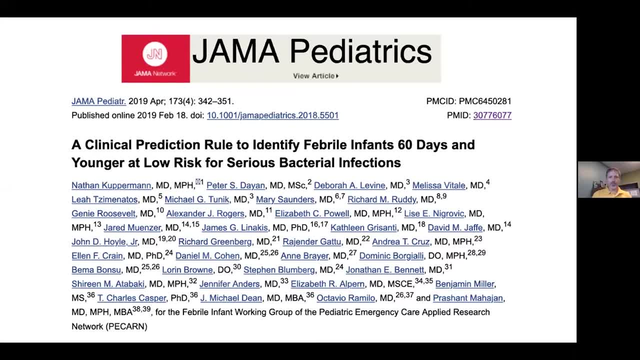 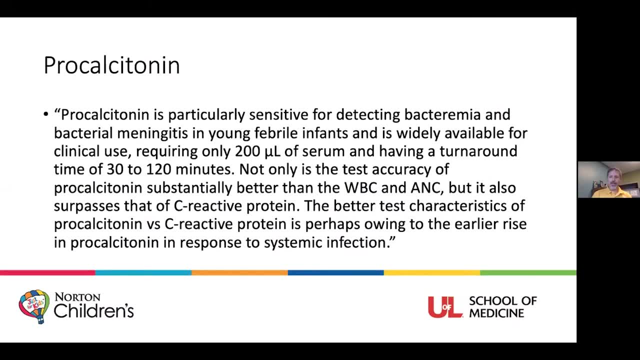 febrile infants younger than 60 days, and tried to come up with a rule for basically who you had to do a lumbar puncture on. And again, this is again about procalcitonin. This is from that article. Procalcitonin is particularly sensitive for detecting bacterial endotoxins, And so this is. 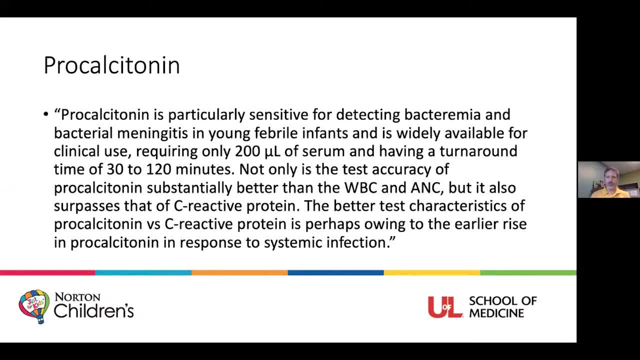 a study done in the US at the University of Colorado a few years ago, And it's very relevant for clinical use. And it's widely available for clinical use, requiring only 200 microliters of serum and having a turnaround time of 30 to 120 minutes. Not only is the test 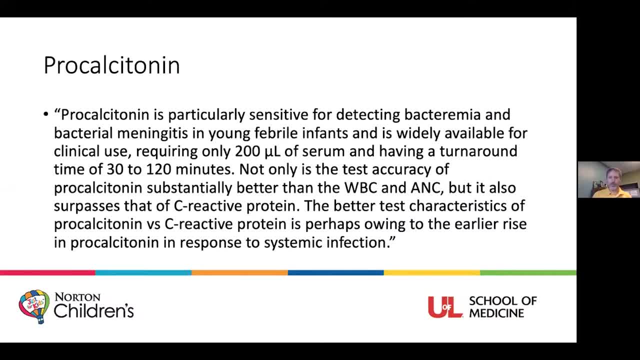 accuracy of procalcitonin substantially better than the white blood count in A and C, but it also surpasses that of C-reactive protein. The better test characteristics of procalcitonin versus CRP is perhaps owing to the earlier rise in procalcitonin in response to systemic infection. 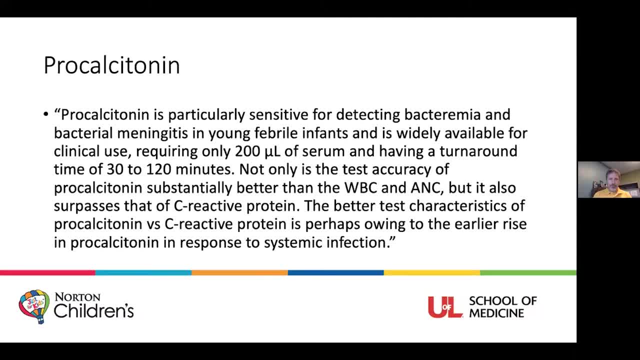 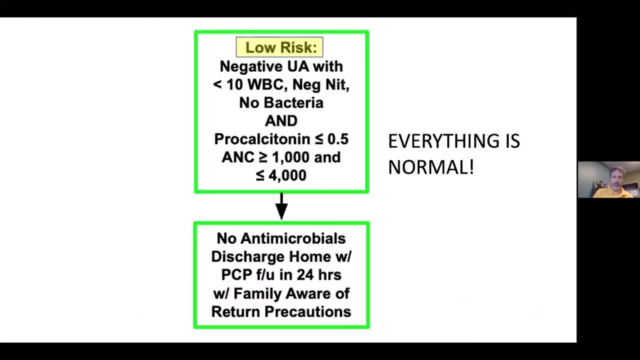 Okay. So these authors- and I'm going to go through this a little bit more- but they thought and believe, based on their data, that procalcitonin is an important marker for sepsis. All right, All right. So getting back to this algorithm, because, remember, we did urine, blood and procalcitonin. So children categorized- and again these are 29 to 60 day olds, categorized as low risk- have a normal urine, a normal ANC and a normal procalcitonin. 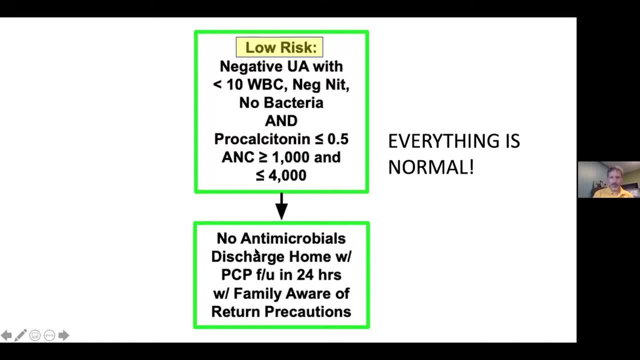 Everything is normal. So those kids who look well go home and we ask that they follow. We ask that they follow up with you, with the pediatrician the next day. So that's a big change from when I trained- I finished residency in 2008.. And from when many of us trained, we're a 35 day old with a fever of 102, like the one we talked about. 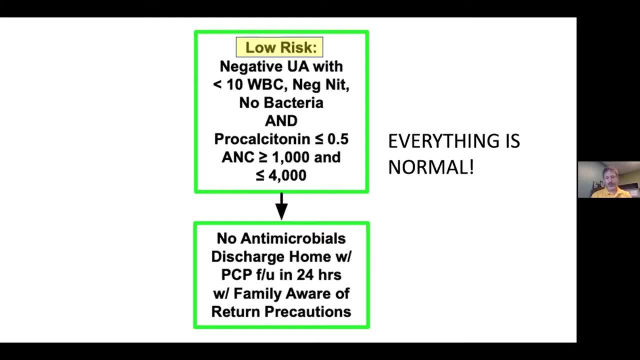 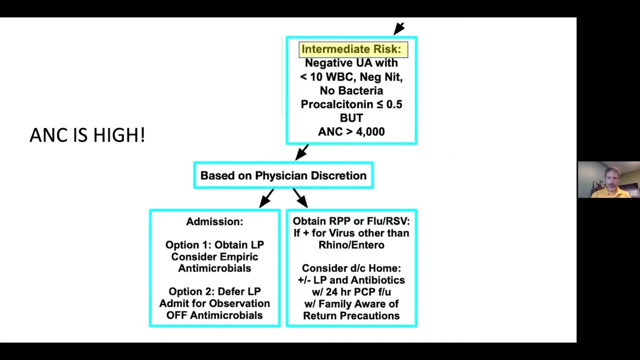 We didn't do procalcitonins then, but they all got lumbar punctures and they all got admitted And again normal procalcitonin. All right, There's an intermediate risk category as well. This is taken directly from that algorithm. 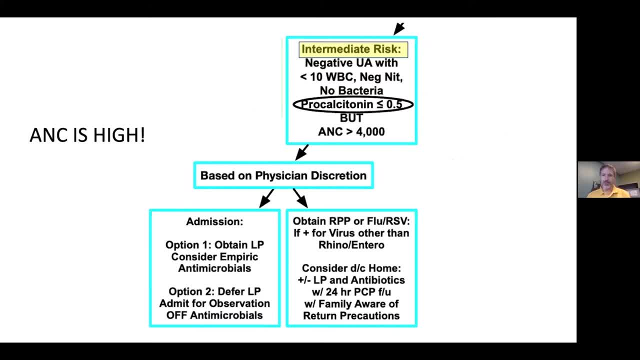 Okay. So again, the procalcitonin is normal, but the ANC is greater than 4,000.. All right, In that case you really have two options. One is to admit them, get an LP and observe them either on or off antibiotics, or admit them not, get an LP and observe off antibiotics. That's this first box. 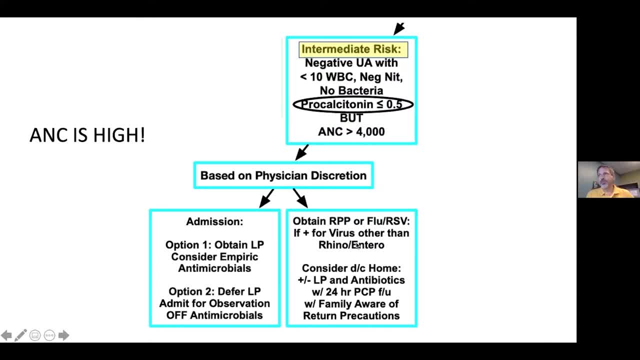 The other box here sort of tries to help you stratify the risk further by looking for other causes of fever And if you find them, consider sending the child home with or without a lumbar puncture, with or without antibiotics, with close follow-up assured. 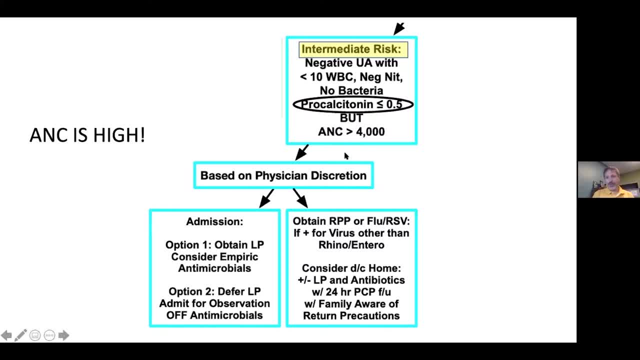 So this intermediate risk category, I will say, is unusual. Usually they're low risk, but then the rest of them are high risk. We don't see the intermediate risk too often, But this is sort of where you know experience and comfort level of how the child looks and what the family really comes in, far more so than in the other circumstances where we have a clear path to follow. 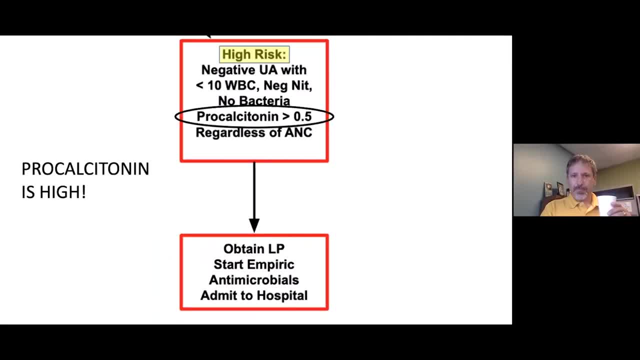 All right. High risk is when the other labs aren't really relevant. High risk is when the procalcitonin is high And these children get treated the same way we used to treat them, Same way we treat somebody During the first four weeks of life, which is we've already gotten the blood and urine. 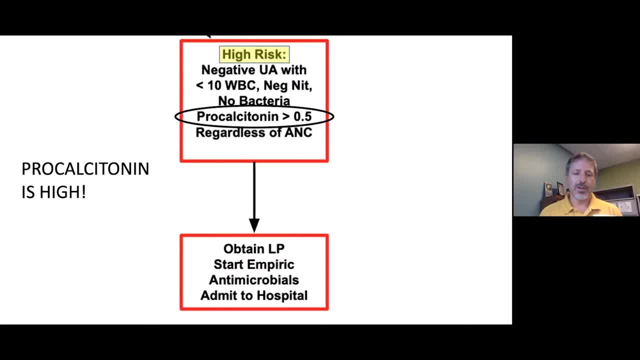 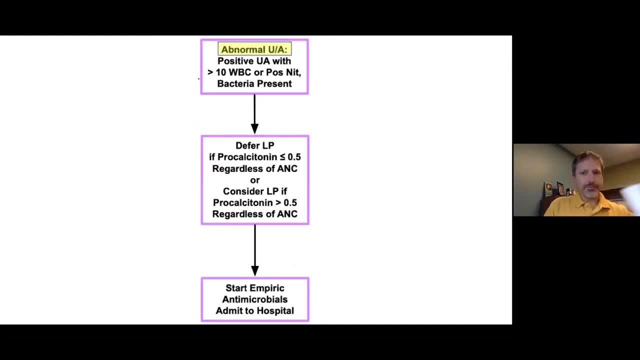 Now we're getting a lumbar puncture, We're starting empiric antibiotics and we're admitting the child to the hospital. And then there's this other category where they have an abnormal UA which, in the way we look at it, is as positive nitrites bacteria present or there's greater than 10 whites. 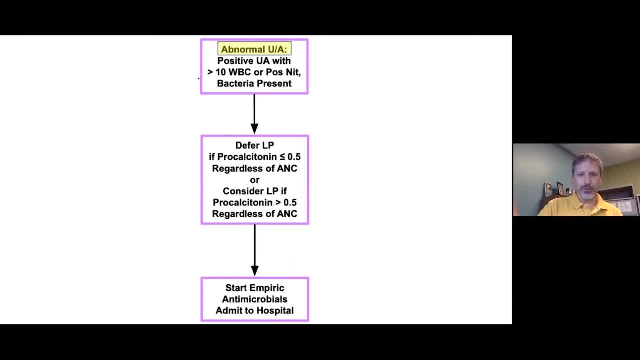 And we would only do these as cath urine. So pretty reliable for those categories. If the procalcitonin is normal, we don't need to do an LP. If the procalcitonin is high, we would do an LP in that case. 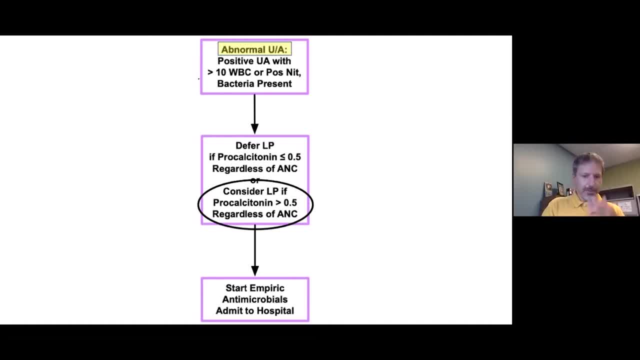 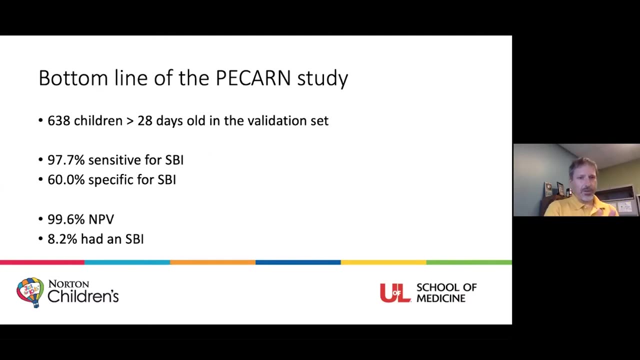 Okay, And then after that those children will be started on antibiotics and admitted to the hospital because they have the SPI- serious bacterial infection, the UTI, All right. So this is that study, The Jammapede study that we talked about, where they use procalcitonin. 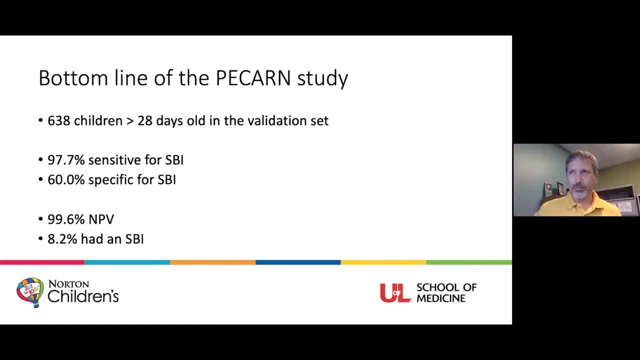 And they basically the algorithm that I just reviewed- mirrors what was done in this study. So there were, in their validation set 638 children greater than 28 days old And they found their rule- the algorithm we just reviewed- to be 97.7% specific and 60%. 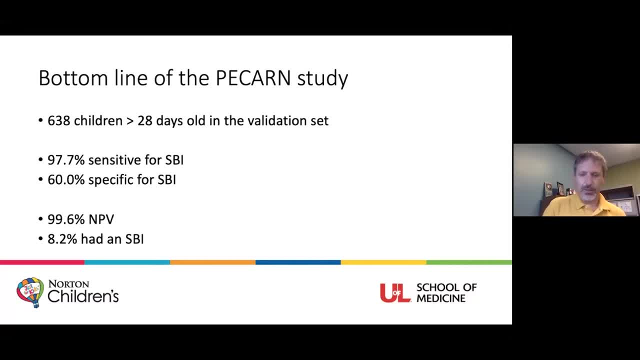 Or sensitive: 97%. sensitive: 60% specific right, And you may remember those are in statistics. sensitivity and specificity are characteristics of the test, They don't change based on the population. And then in their validation population, the rule had a 99.6% negative predictive value for SPI. 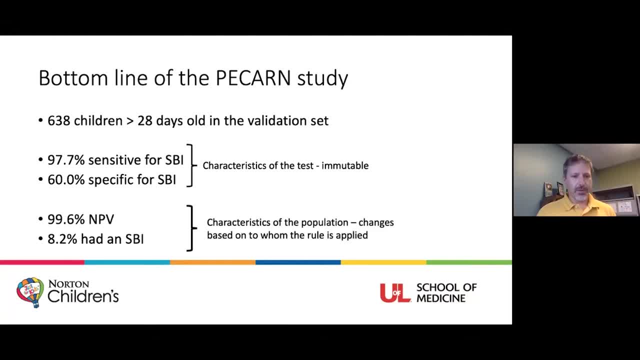 And that is a characteristic of the population. So in their population, 8.2% And 5.2% of the children had an SPI, and of those, they missed two. We'll talk about that in a second, Because this study was based on a sample of emergency departments across the country and was gathered prospectively. it's very powerful. 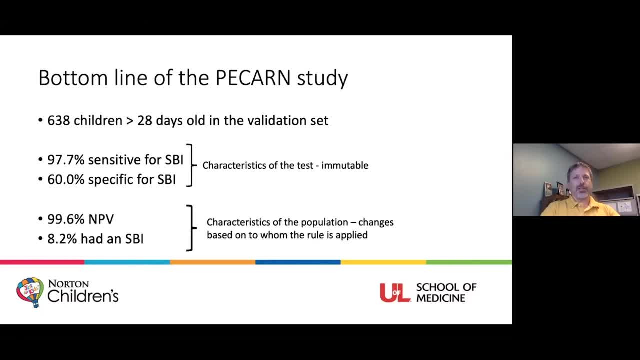 And we think- and this is the collective, we pediatric emergency medicine people think that this population mirrors our own population, So it's a good rule to apply in our population. So you note that it's not 100% sensitive, that the negative predictive value is. 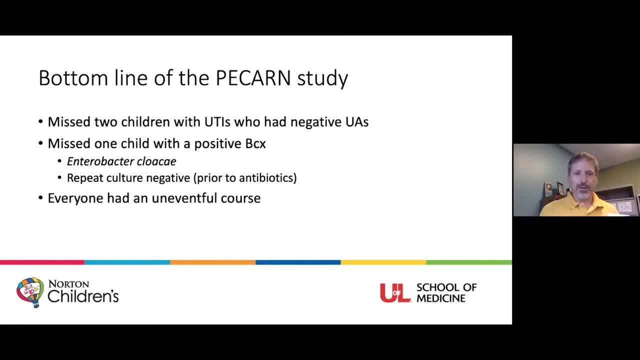 not 100%. So what happens? So they missed two children who had a UTI. Both of those kids had a negative UA. And then they also missed one child who had a positive blood culture which appears to have been a contaminant As a repeat culture. that was done prior to the child getting. 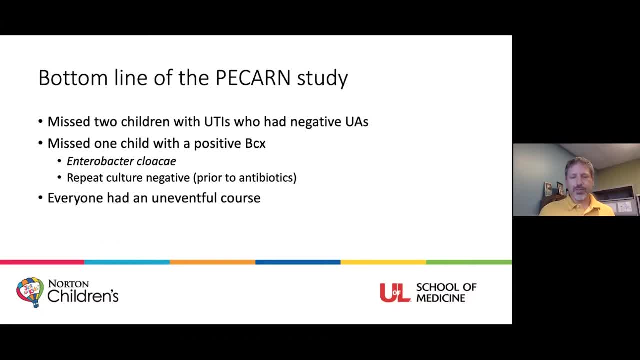 antibiotics was negative. Either way, all of these kids had an uneventful course. So that's pretty powerful stuff And that's why this and this isn't just locally. this is sort of this wave has swept the country. This is why we do the evaluation of febrile children greater than 28. 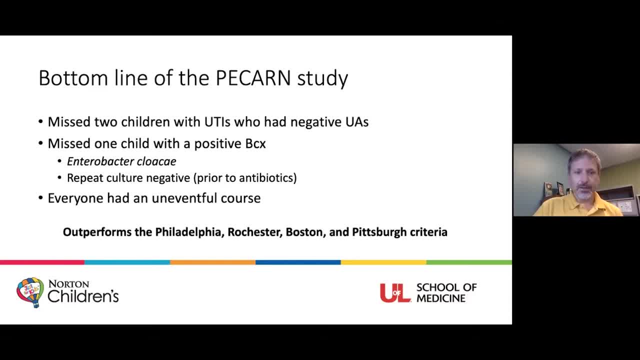 and less than 60 days in this manner, And notably those. so those test characteristics outperform the criteria we all learned when we trained. So Philadelphia, Rochester, Boston. I was in Pittsburgh, it was a Pittsburgh criteria. It outperforms all of those. It's a better rule. 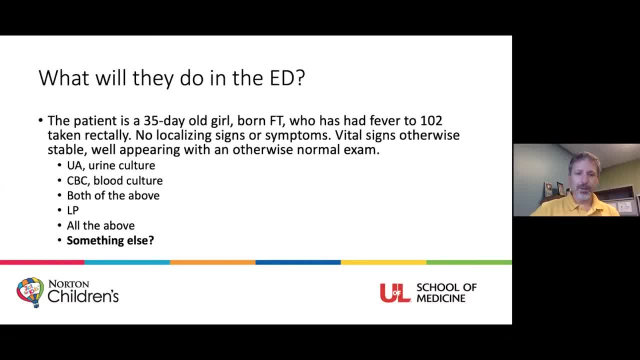 a better algorithm, All right. So what will they do in the emergency department for this patient? Well, it's obviously the something else, because we would do the first two, A and B or whatever, and then we would do a procalcitonin in addition. 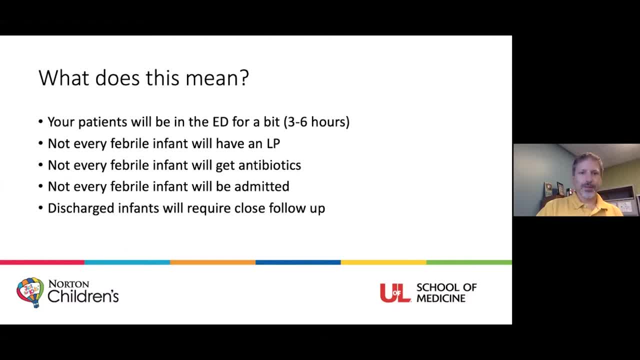 Uh, there you go. What I just said, All right. So what does this mean? You know, this stuff takes time, And so when you send a patient to me in the emergency department, that falls into this algorithm, they're going to be in the emergency department for a little bit because we have to get the data. 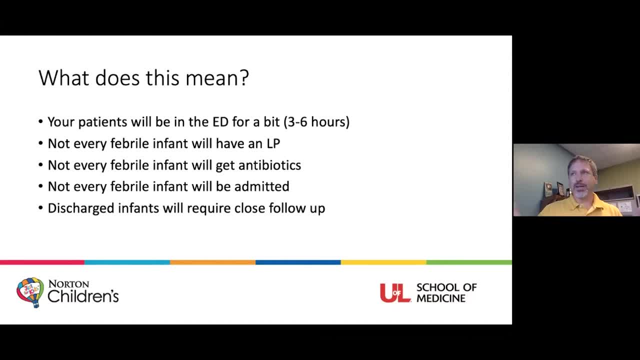 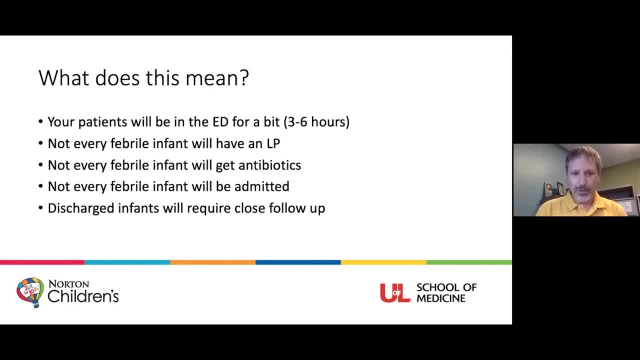 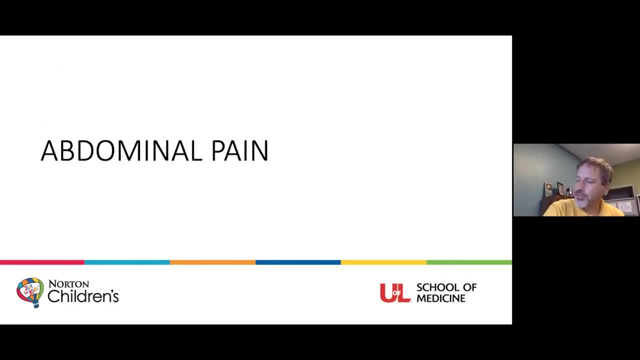 give out the data. We don't give out the data. We don't give out the data. We don't give out the antibiotics to every single one of them. We don't admit every one of them And the ones that we don't admit that we discharge. we rely on you for close follow-up, All right? So, uh, as I said, 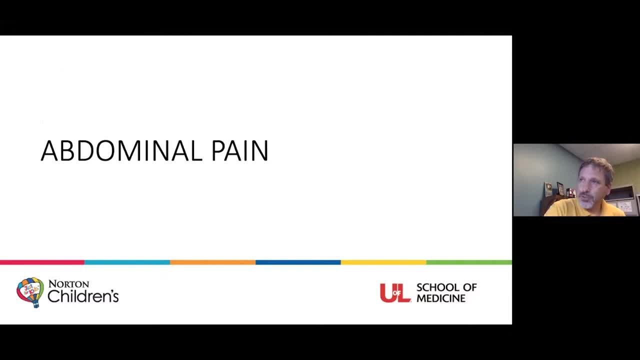 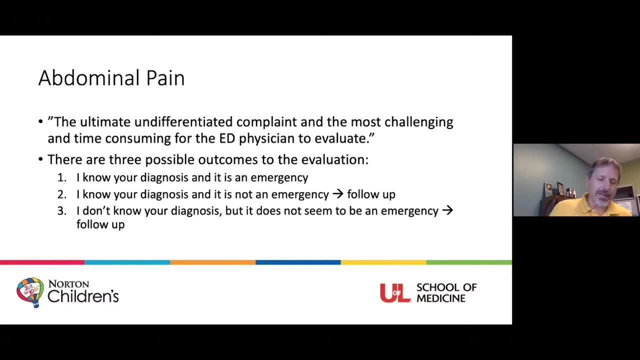 that was the easy one, right, Because we have really good data and we have very objective measures of everything. We're going to move on here to abdominal pain. I can't remember who told me this, But uh, they said that it's the ultimate undifferentiated complaint and the most. 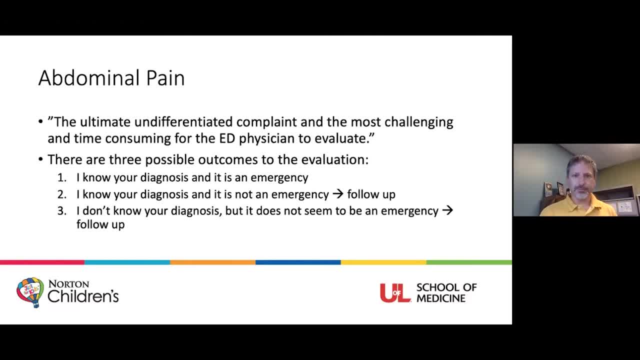 challenging and time-consuming for the ED physician to evaluate. From my perspective, there are three possible outcomes to this emergency department evaluation. You show up, I see you. I either know your diagnosis and you're having an emergency and we need to admit you do an operation, give antibiotics whatever it is, or you show up, I see you. 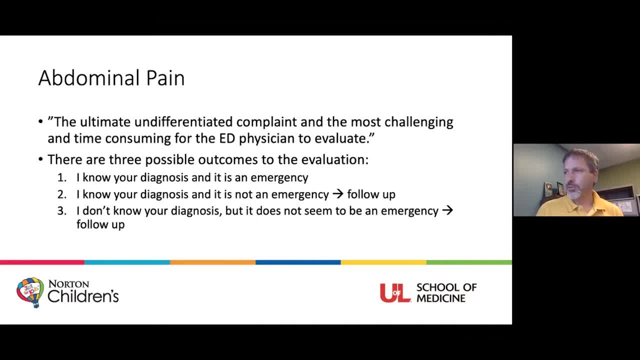 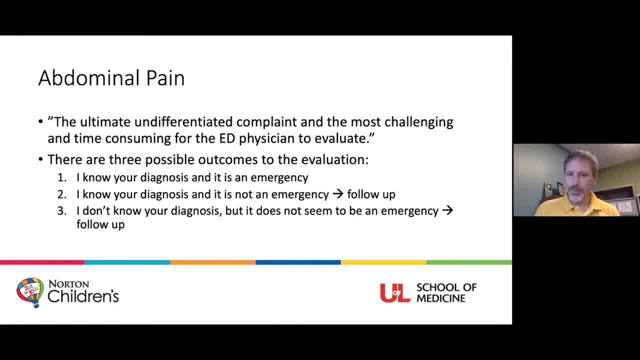 not exactly sure what your diagnosis is, but it doesn't seem to be an emergency. but you can safely be discharged and you'll need to follow up. So those are the possible outcomes And we see those outcomes, you know, commonly every day when we're working All right. So why has the 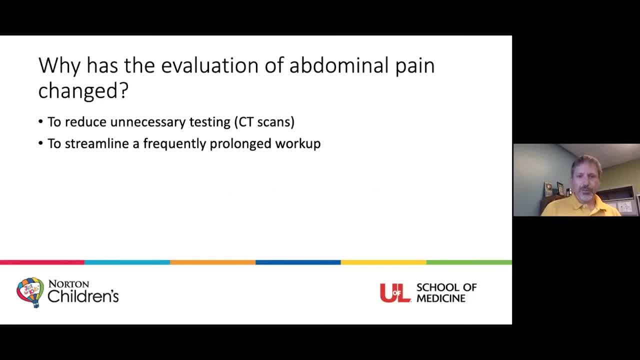 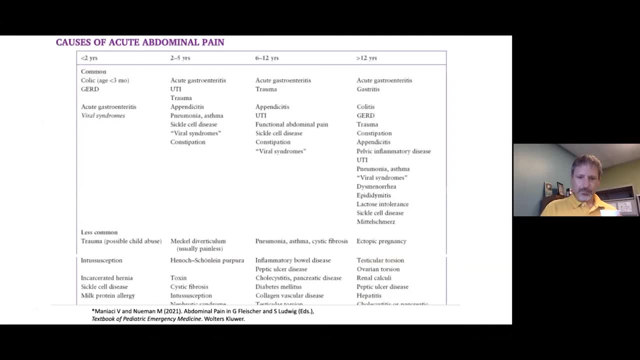 evaluation of abdominal pain been so challenging. Well, it's because we don't know what your diagnosis is. It's really to reduce unnecessary testing, particularly CT scans, and to streamline the way we do a workup that's really frequently performed. So this is from Fleischer and Ludwig. 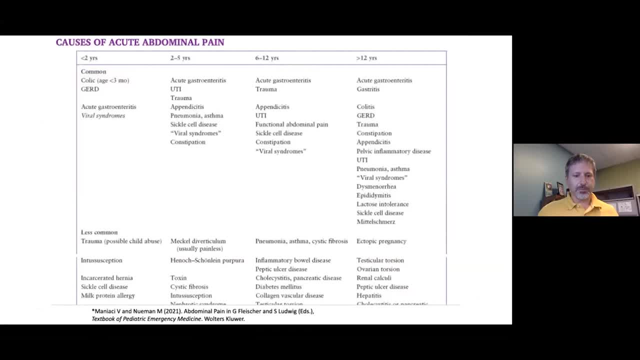 and I'm just showing this as an example. So Fleischer and Ludwig is the textbook of pediatric emergency medicine. It's our Nelsons, And this is just a portion of a table on one page that shows me all the causes of acute abdominal pain. And I'm just showing this as an example And I'm just 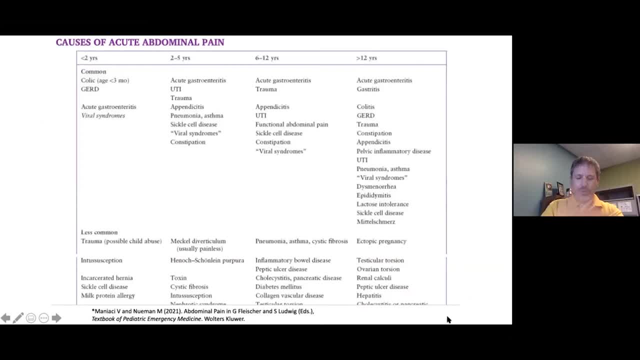 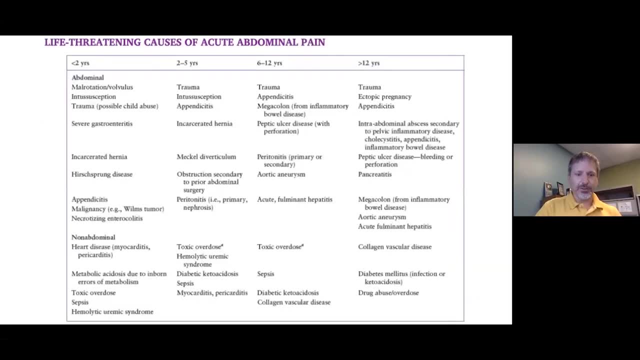 showing this as an example. So Fleischer and Ludwig is the textbook of pediatric emergency medicine And I'm just showing this as an example. And I'm just showing this as an example And I'm going to show all of that. My point here is that abdominal pain has a broad differential diagnosis. 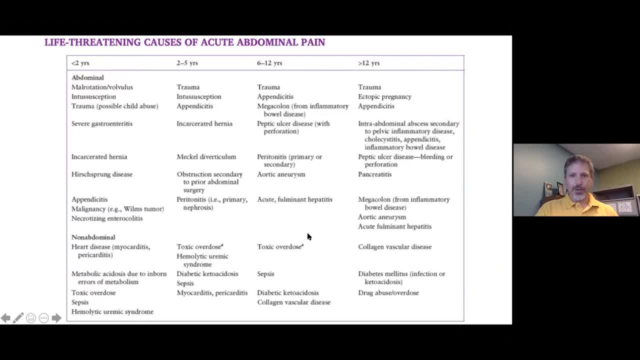 And then same textbook. they tried to tell me the 30 or 40 things that I would need to figure out immediately because they're life-threatening causes of acute abdominal pain. Again very broad ectopic: pregnancy, aortic aneurysm, incarcerated hernia- you know all these different things. 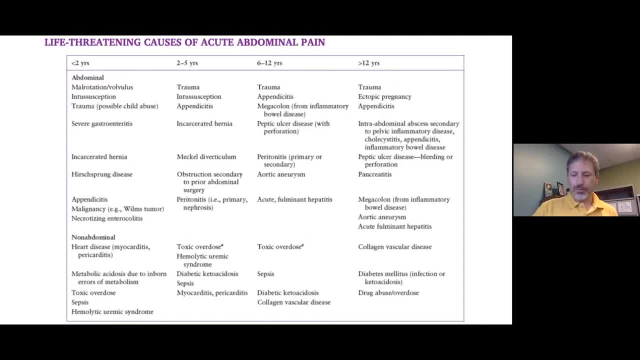 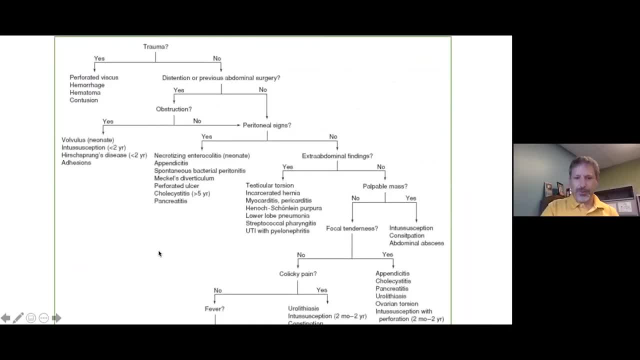 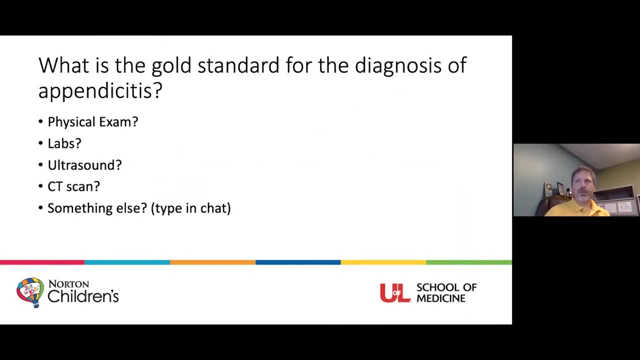 to break this algorithm down. You can see- and this again goes on for three pages- It just kind of, you know, continues on and on and on and on, Very challenging, And so this is really something that we wanted to streamline. So we have a poll question, though So frequently we get sent. 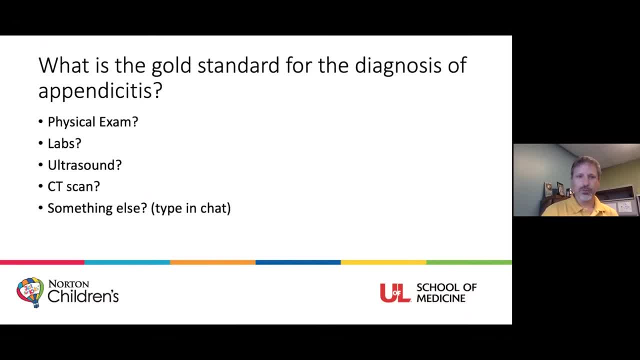 patients or see patients who were concerned for appendicitis. So what is the gold standard for the diagnosis of appendicitis? We'll give that a minute or two or a few seconds. I guess I just made my vote All right, Gold standard. So a third said physical exam, a little over. a third said: 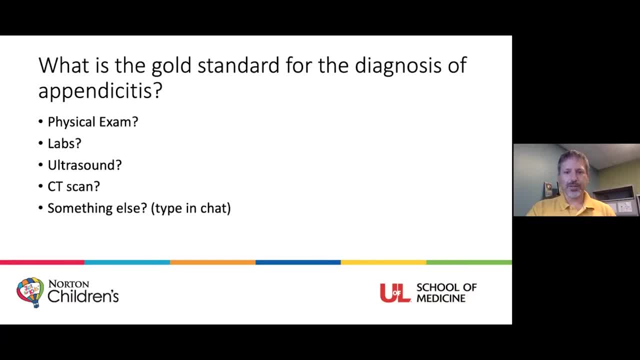 CT And then some folks thought some labs and ultrasound And so all good guesses. but you know, you probably guessed that it's not going to be quite correct. So you know I asked: Cindy Downard is our chief of surgery here, chief of pediatric surgery. So what is the gold standard? 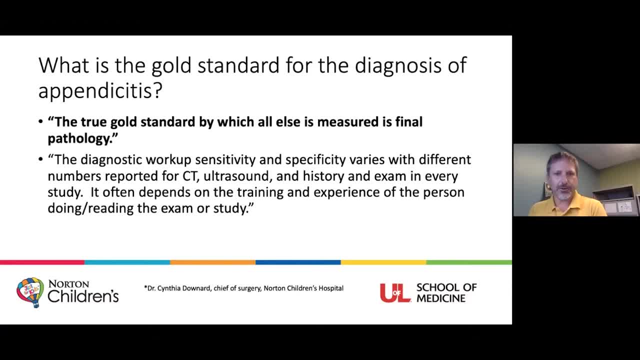 for the diagnosis of appendicitis, And this is her quote. to me, the true gold standard by which all else is measured is spinal pathology. It means you do the operation, take the appendix out, slice it up and look at it under a microscope. 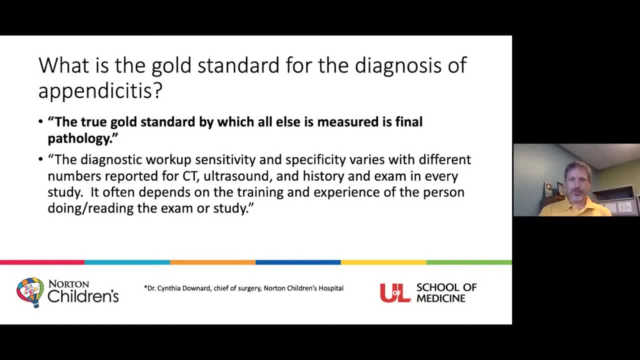 She said the diagnostic workup sensitivity and specificity varies, with different numbers reported for CT, ultrasound and history, and examine every study. It often depends on the training experience of the person doing slash reading, the exam or study. And that is very true. We'll talk. 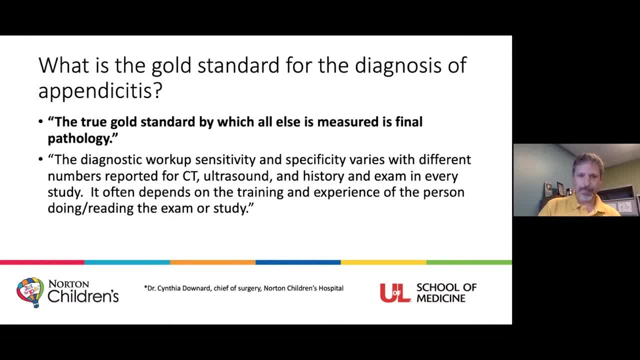 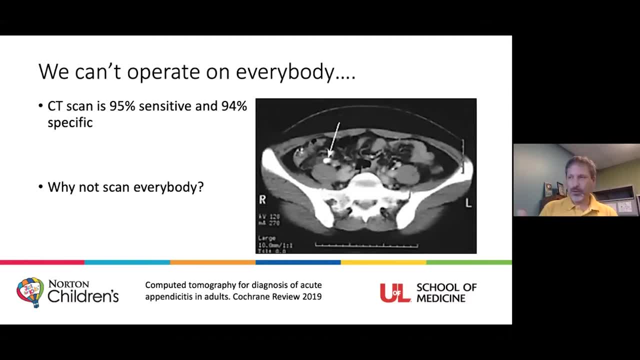 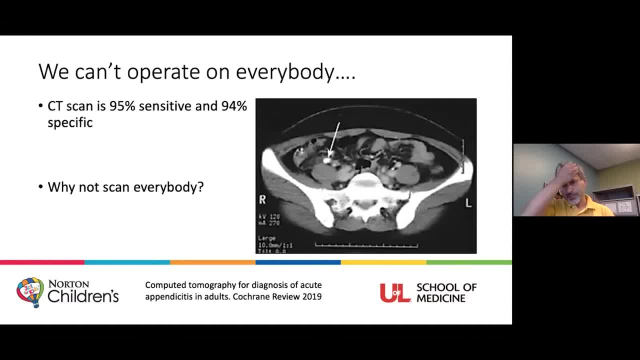 take off, We're going to take off, We're going to take off, We're going to take off. We got your appendix and look right, We can't do that. So we you know, CT scan is maybe the next best thing. This. 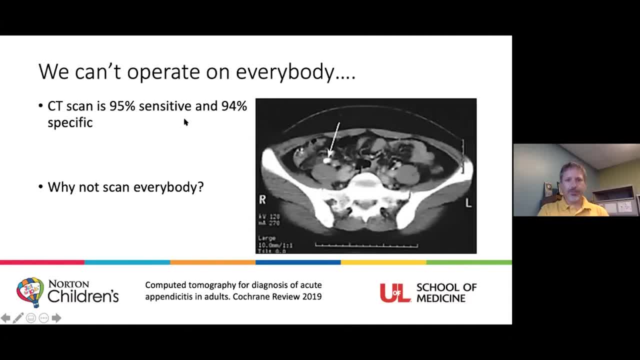 is from a Cochrane review from a couple of years ago. It's 95% sensitive and 94% specific. That's for appendicitis. Okay, That's pretty good, And this is that's. that's actually an appendical. 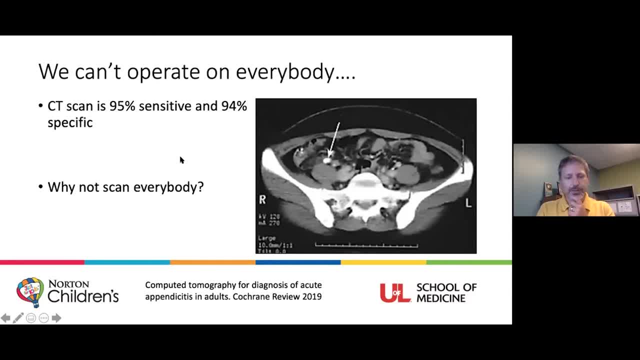 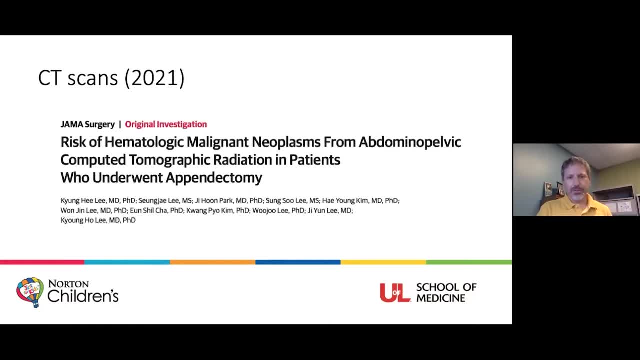 lith there So that one's pretty obvious to read. You can probably see that on a plain x-ray, actually, But at any rate. so why not just do CT scans on everybody? That's an interesting question. So this is a study that came out, I think, in February of this year, and it's a 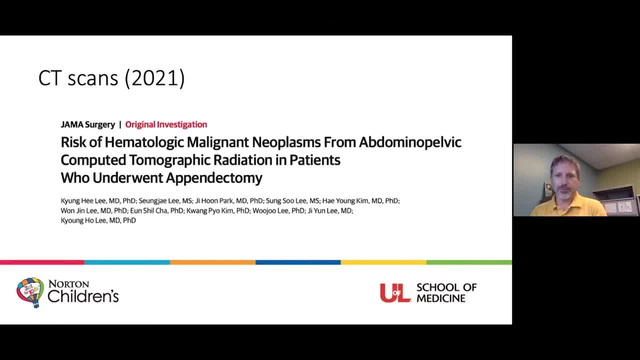 pretty good one. So risk of hematologic malignant neoplasms from abdominal pelvic computed tomographic radiation in patients who underwent appendectomy, which is a mouthful. It was a Korean study and they did a retrospective look over many years of everyone in their system that 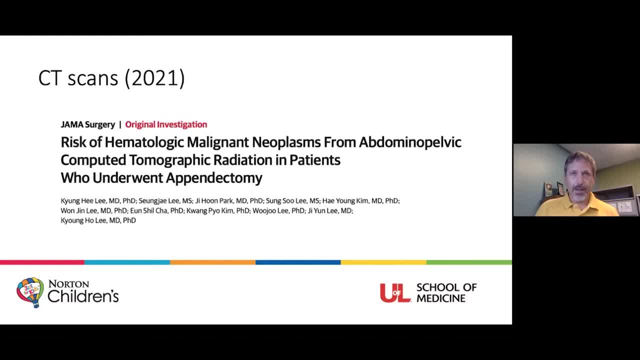 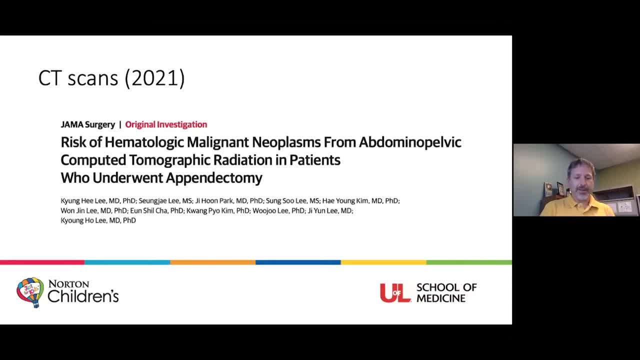 after that, their appendectomy. So, basically, did they have a CT scan and then get their appendix out, or did they just get their appendix out? Okay, That's what they looked at And this was all comers- adults and children- And so this is from their discussion, And I highlighted the part. 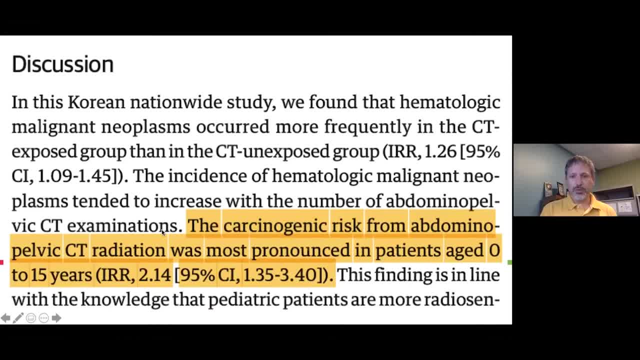 that, I think, is important. The carcinogenic risk from abdominal pelvic CT radiation was most pronounced in patients. The carcinogenic risk from abdominal pelvic CT radiation was most pronounced in patients, And so that's what they looked at, And so this is from their discussion, And so this is from their discussion. 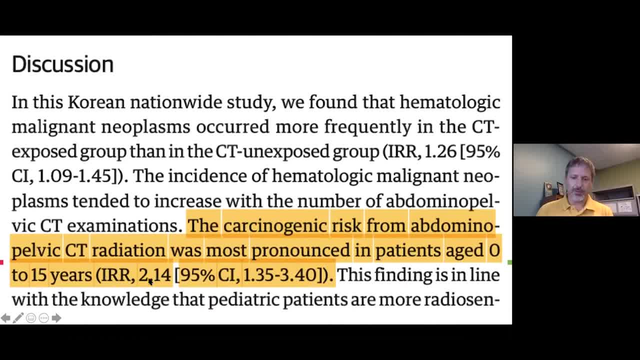 And the risk ratio was 2.14.. So, and it was mostly leukemias, not solid tumors, It was mostly leukemias, but basically you are twice. the group that got a CT scan prior to the appendectomy was twice as likely to develop an oncologic process, Mostly leukemia was twice as likely to develop. 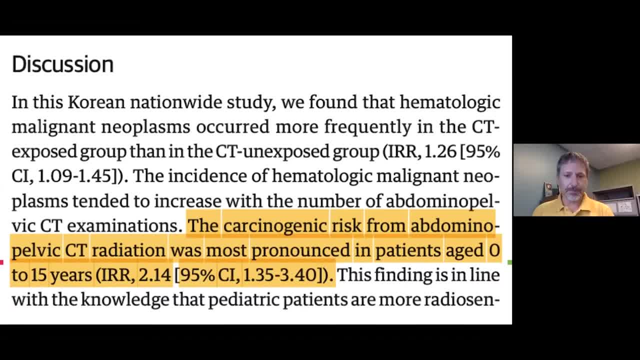 that at some point in their life, compared to the group that didn't get a CT. That's really profound data if you're me, because you see a lot of kids with belly aches and I got a CT scanner right down the hall, right, So I really need to be thoughtful about who I'm scanning. 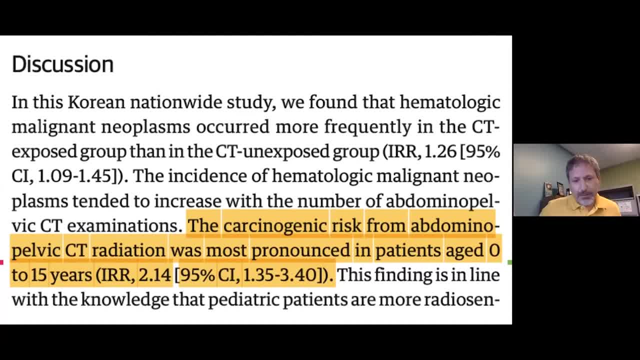 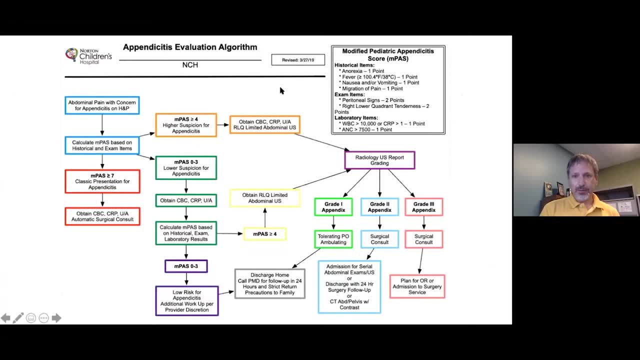 and to try to minimize that, because I could have potentially could be ordering a lot of CT scans and doubling someone's risk for leukemia certainly isn't consistent with what I want to be doing as a doctor, So that's why this is important. So, again, we have this appendicitis evaluation. 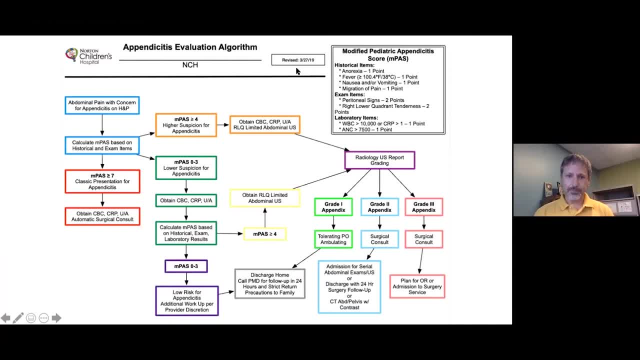 algorithm. This is from 2019.. All right And the same. we're going to do the exact same thing. We're going to break this down into pieces. Stay with me. So we're going to start up here. So notice that first blue box says abdominal pain with concern for appendicitis on HNP. 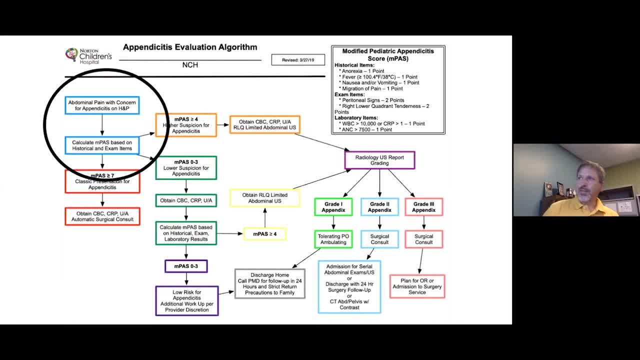 So that means they have to be telling me the right story. The story can't be that I haven't had a bowel movement in two weeks and my whole belly hurts. That's not appendicitis. We don't think about it that way And I would approach that differently. 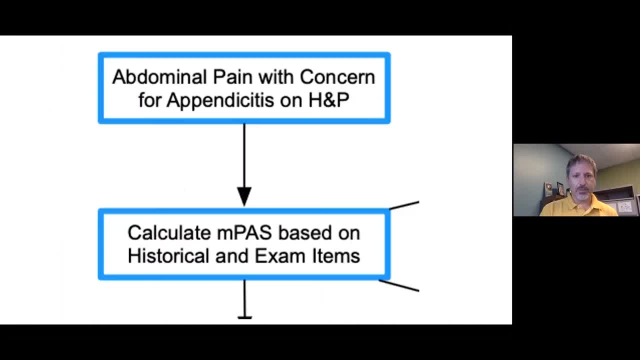 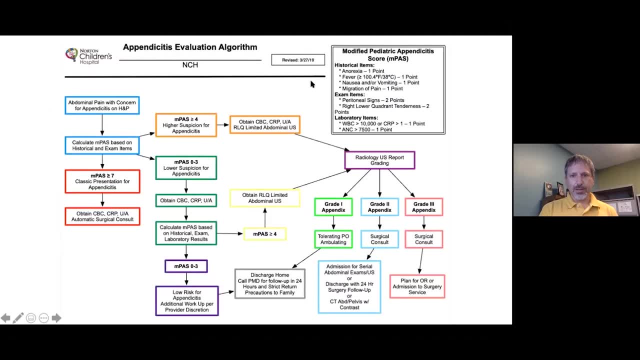 So it has to be a consistent story. And then what we do- again it has to be a consistent story- is calculate this MPAS. Okay, And MPAS is up here. I'm going to focus in. right, Am I focusing? Yes, 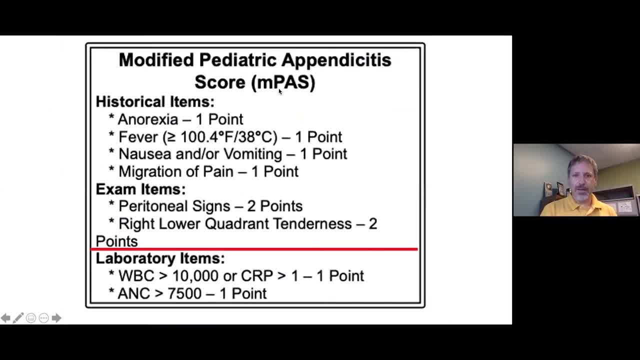 I'm going to focus in on it. So MPAS- modified pediatric appendicitis score, All right, And we're going to calculate that based just on the history and physical exam items. So the things above this red line that I put here, So do they. 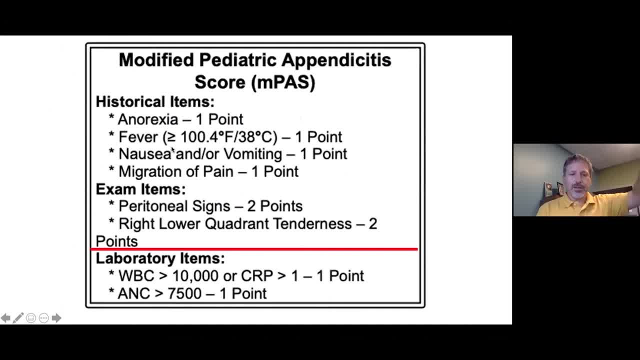 have a history of. so these are all things that we would think of as classic history and physical exam items, classic for appendicitis. So they have anorexia, they have a fever, they have nausea or vomiting. Do they have migration of their pain? right? We usually think. 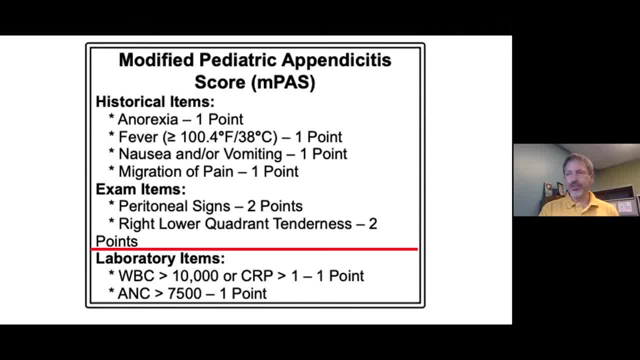 peri-umbilically to the right lower quadrant And then on exam, do they have peri-umbilically to the right lower quadrant? Do they have perineal signs like rebound? And do they have right lower quadrant tenderness? All right, And you can see points are assigned to each of those, So right. 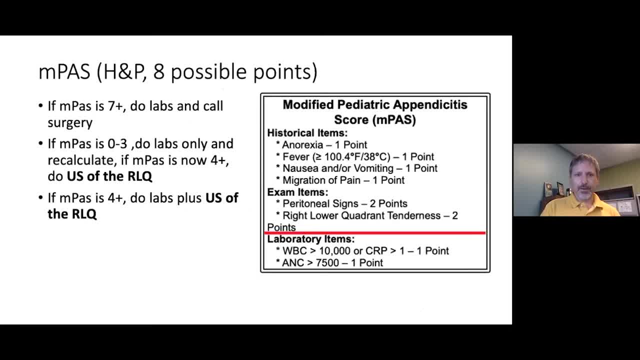 now we're only looking at what's above the red line. All right, So on that portion there's eight possible points. Okay, If the score is seven plus seven or more, we're going to do these labs, CVC and CRP, And then we're also going to. 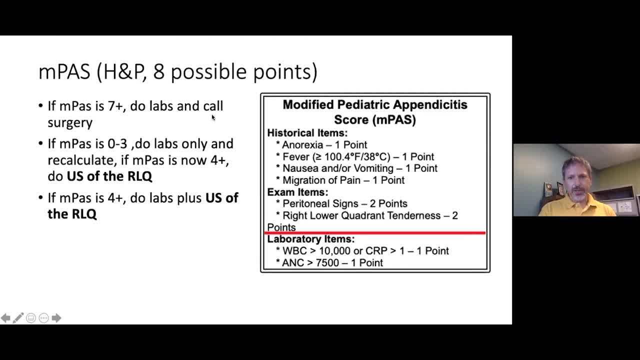 um, uh call surgery in that case. Cause the. the idea is that this sounds like a classic story. history and exam for appendicitis Surgery should just come and lay a hand If the MPAS score is zero to three. again just based on the history and exam items. 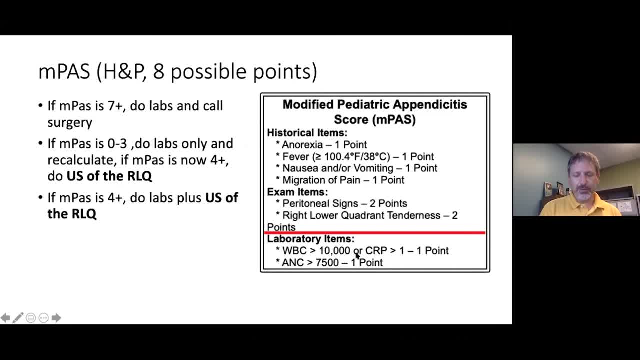 we do the labs, So we do these, And if that gets them up over four, we're going to do an ultrasound of the right lower quadrant. Okay, If the score is four, really four to six, we're going to do the labs again And we're going. 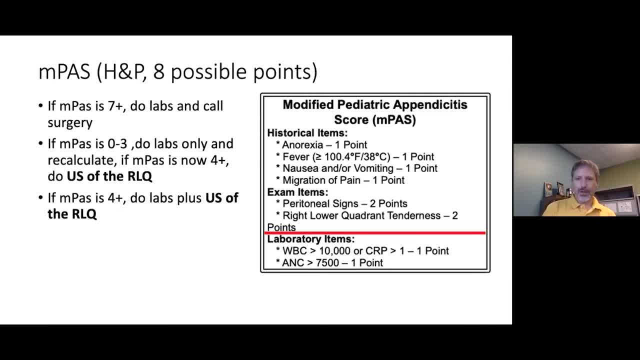 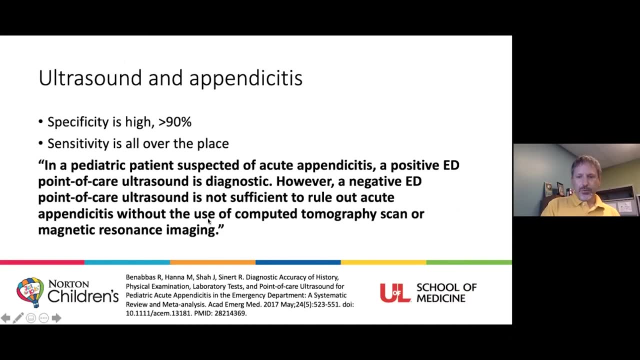 to do this ultrasound of the right lower quadrant. All right. The reason we're saying ultrasound, of course, is because there's no ionizing radiation there. We don't want these kids to wind up with leukemia, All right. So, uh, this is uh from a study that really looked at, um, uh. 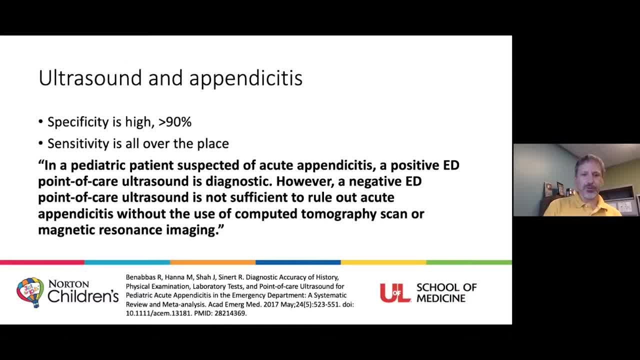 bedside point of care, ultrasound for appendicitis, but the numbers are pretty similar for um, uh, when the radiology does the ultrasound, which is how we do it here, We would send these children for formal ultrasound with our ultrasound texts. So the specificity is high. If you see an abnormal, 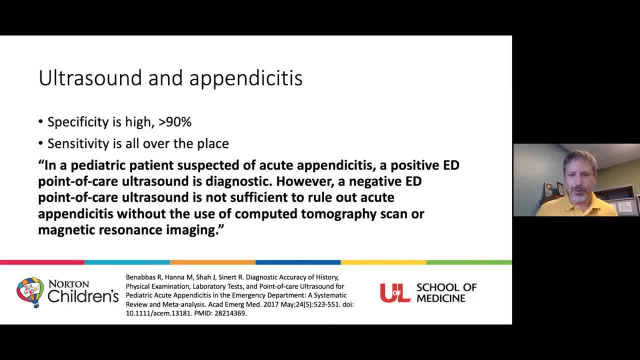 appendix. it's appendicitis, but the sensitivity is all over the place, Um, so you can see here: positive ED point of care Ultrasound is diagnostic. However, a negative ultrasound is not sufficient to rule out acute appendicitis. So we're going to do this ultrasound with our 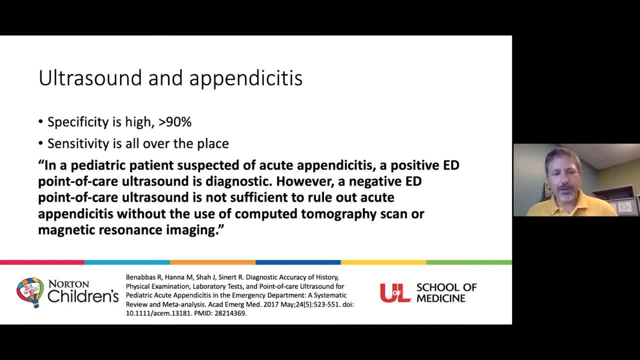 patient. So we're going to do this ultrasound with our patient. So we're going to do this ultrasound without the use of an CT scan or MRI. Um, the uh sensitivity really varies based on the habitus of the child. Uh, so children with more adipose tissue are more difficult to 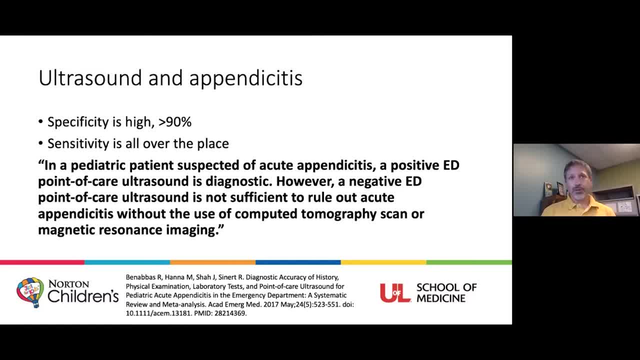 get to the appendix, Essentially, when you're looking with ultrasound, it also depends with on how um, how good the ultrasonographer is, how familiar they are with this particular study. Ultrasonography is like any other skill: The more of them you do, the better you get. 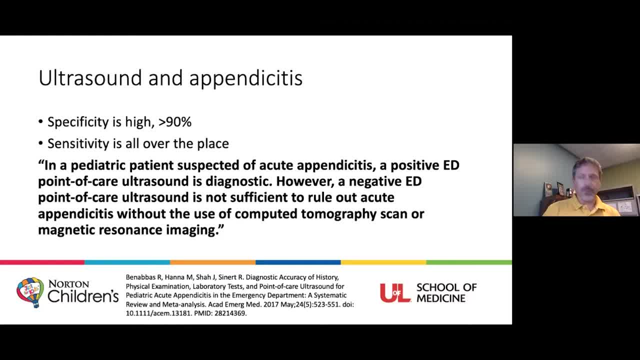 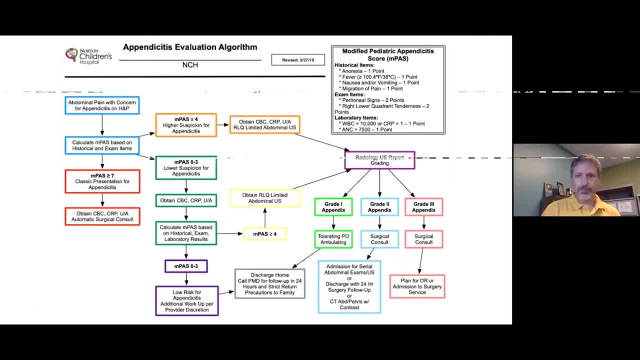 And so we have, uh, some ultrasonographers who do this study more frequently and have done it a million times and they're better at it than those who are novices. All right, So, uh, we've walked through and we're over here now. uh in, uh, really, what these ultrasound results are. Okay, 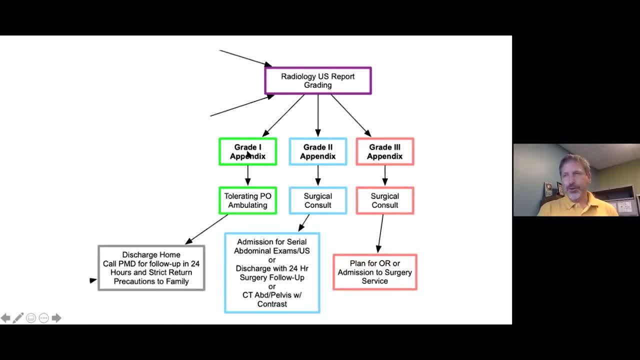 So these ultrasounds are graded. I don't know where this grading system came from. I believe it's internal. So we have grade one, grade two, grade three, Grade one is a normal appendix is seen. So that means we saw the appendix. It looks fine. We PO challenge a child. They're walking around. 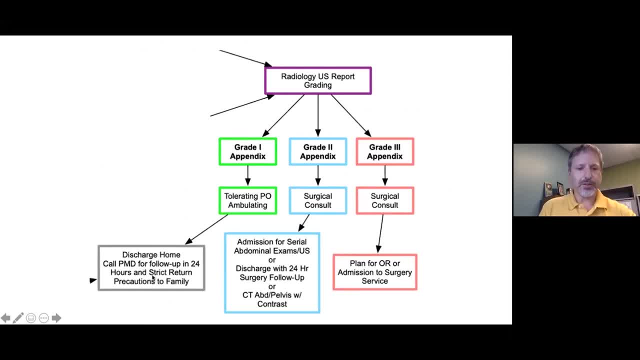 We discharge them home. Hope they follow up with you in a day or so. I explained to the family reasons to return. Of course, that's grade one. Grade three is: we see appendicitis. So we found the appendix and it's abnormal. Uh, and in that case we're obviously going to talk to surgery. 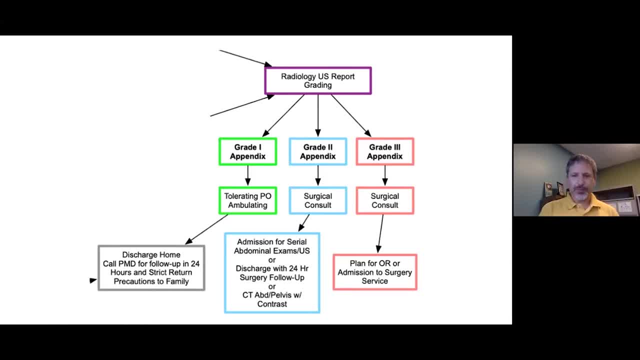 And defer to them, and they'll do. you know what they do. Of course, grade two is the most common finding, which is we don't see the appendix. essentially, When that happens, we get a surgical consult and then surgery tells us what to do, So they might say: we're going to admit this child. 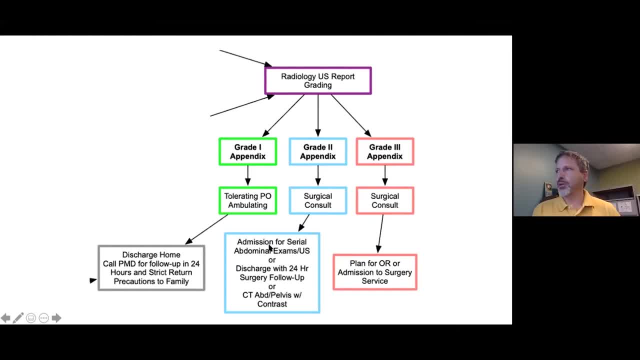 to the hospital. We're going to do serial abdominal exams, maybe repeat an ultrasound in six hours or a day or whatever, and see if this evolves. or we're going to discharge them and we'll see them in 24 hours. Or, you know, we're going to do a surgical consult and we're going to do a surgical. just go ahead and do the CT scan. We don't know what's going on, All right. And I will tell you this: this discharge with the 24 hour surgery follow-up, I've never actually seen them do that, So it's usually either one or the other. They're either going to admit the child and see what. 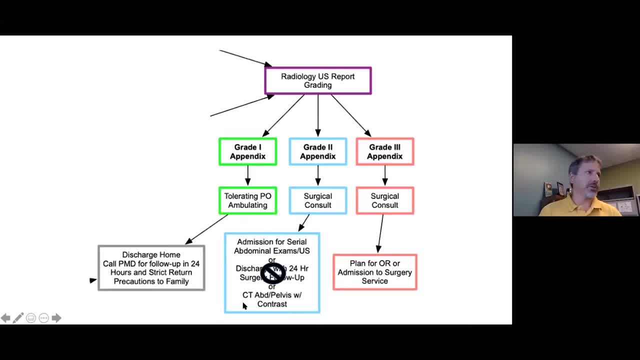 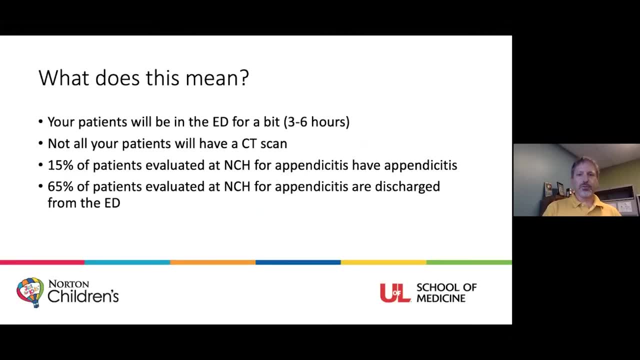 happens or we're going to do a CT scan and hopefully get a reasonably definitive answer in that case. So what does this mean? Again, abdominal pain. it takes time to evaluate. You see, we're getting, we go and see the patient, We're going to do a CT scan and we're going to 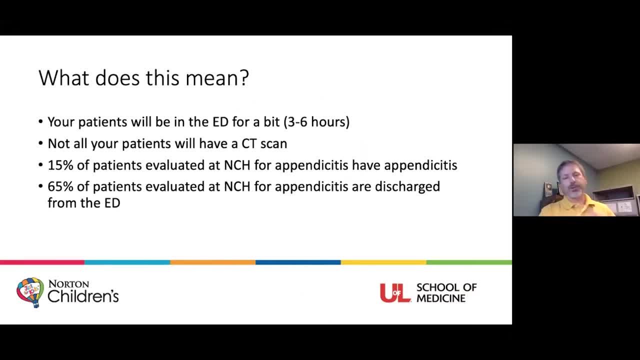 get some labs, Then we're getting an ultrasound, Then we're going to talk to surgery, Then maybe we're going to CT scan. It takes time, Okay, So they're going to be in the emergency department. Not every patient is going to have a CT scan that comes in for evaluate for appendicitis. I will tell you, in the last year or so really, since this algorithm kind of rolled out, 15% of patients evaluated here for appendicitis actually have appendicitis. So that means 15% of patients who go into that algorithm that we just reviewed. wind up spitting out with appendicitis. at the end, 65% of patients evaluated for appendicitis are discharged from the ED, which I think is pretty good. So two thirds of the kids that again enter that algorithm wind up going home. 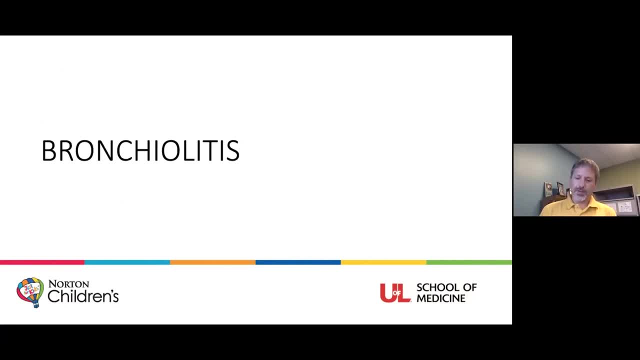 All right, we made it, So now we're going to move on here to the last thing I want to cover today, and that's bronchiolitis. So I I this one of the three things we were discussing today. I think this is the most challenging to. 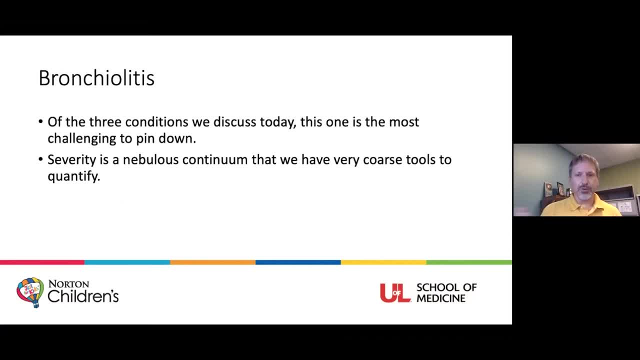 pin down, because the severity is a continuum And the the way we quantify what that severity is. it's just, in my opinion, the tools are very coarse, So why do we even have an algorithm? So we're trying to predict which children need to be. 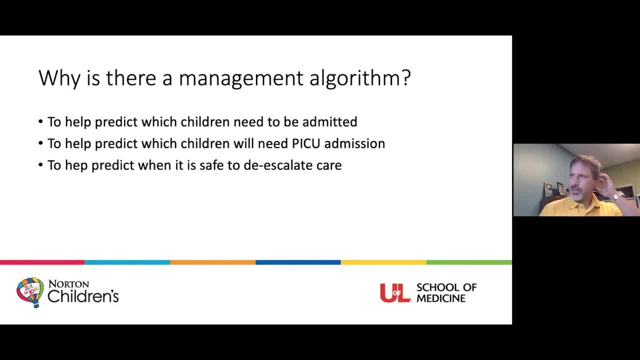 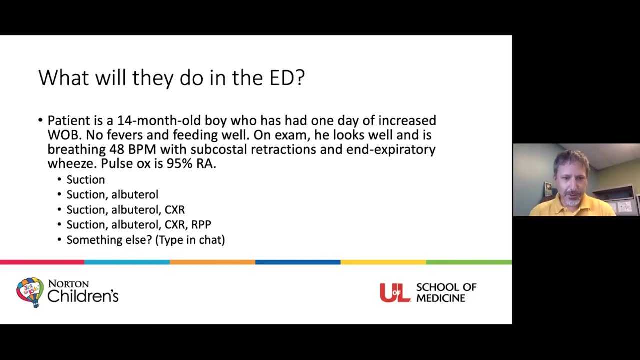 admitted, which children need to go to the ICU And also when it's safe to deescalate care, which children have been admitted and are better enough that we can start taking things away And trying to normalize them. All right, here we are. What will they do in the ED? This is another poll. 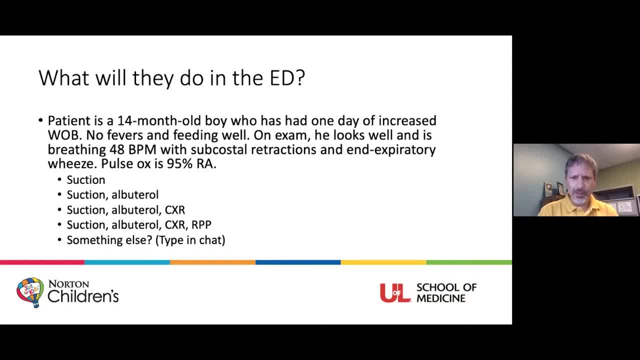 Might be the last one. So we have a 14 month old boy. one day of increased work, of breathing, no fevers. he's feeding well. On exam he looks okay, but he's breathing 48 times a minute with subcostal retractions and inexpiratory wheeze. False ox is 95%. What are we doing in the ED? 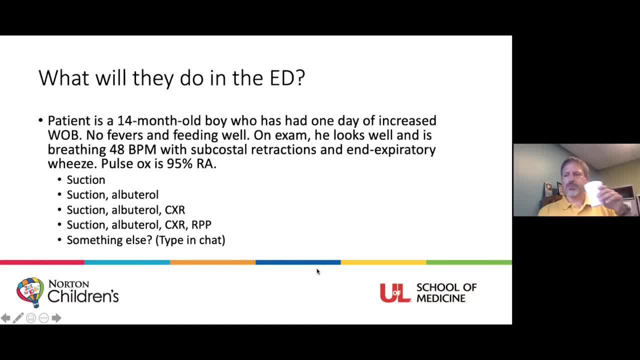 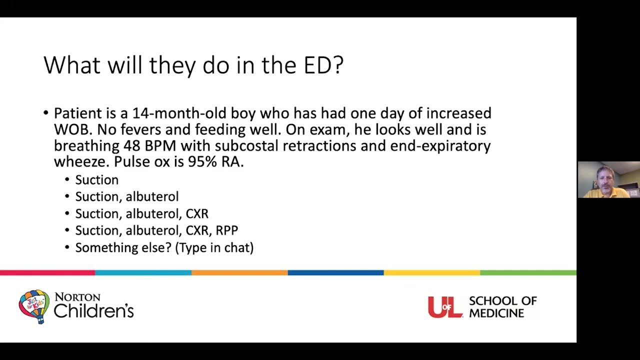 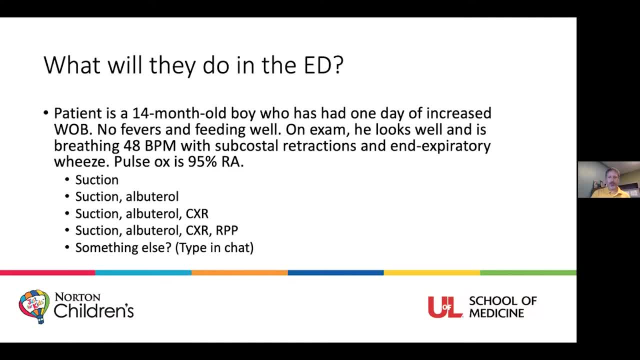 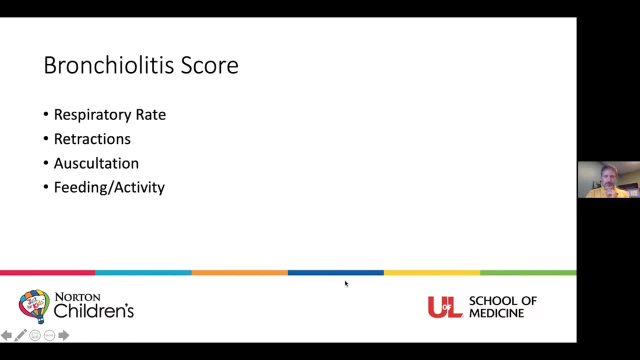 like. the majority went with suction, albuterol chest x-ray and RPP, and then 13% said something else. I can't see the chat, unfortunately, Hold on. No one's typed in the chat, so if anyone wants, 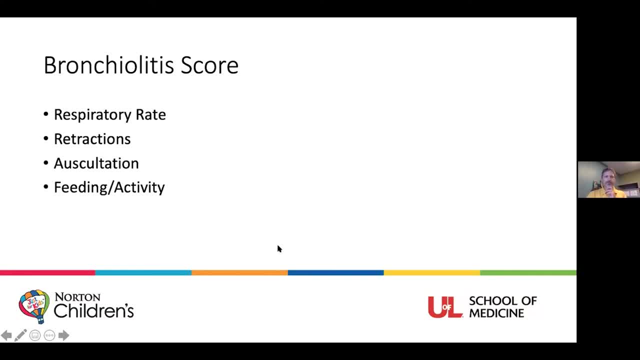 to enter their responses. Okay, fair enough, So something else. but they didn't want to suggest what it was. I guess That's fair, All right. Well, it turns out we have this bronchiolitis score that looks at respiratory rate, retractions, auscultation, feeding activity. I'm going to go. 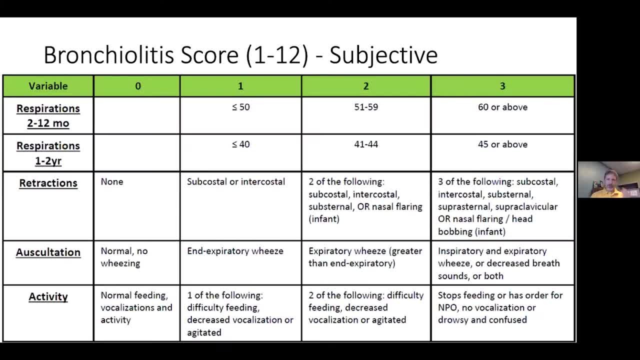 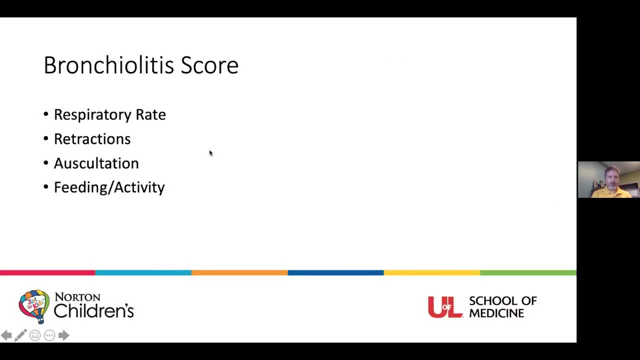 through this so that you understand. Here's this very subjective, or mostly subjective, bronchiolitis score. You can see that part of it varies based on the patient's age. Younger children have different respiratory rate requirements. That's what these are. Sorry about that. 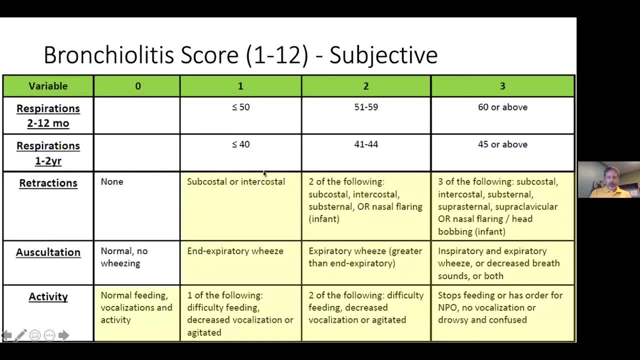 Then older children, children, All right. So, and when I say it's subjective, the what I just highlighted there in yellow, you know, is it end expiratory wheeze or greater than end expiratory wheeze, And some. 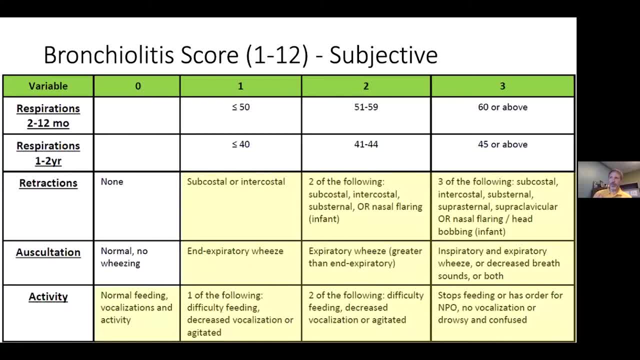 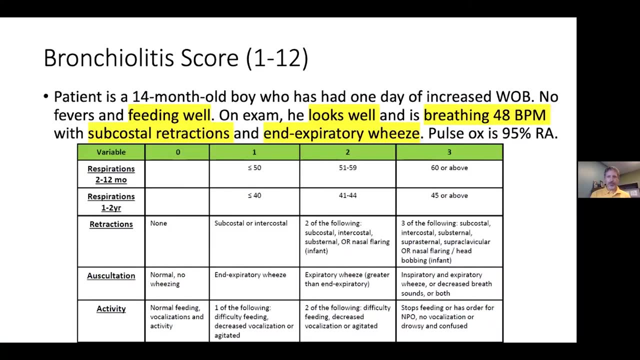 of this stuff is just very hard to um to really pin down And the the reliability of these scores is not as great as I would like it to be. Okay, But at any rate, this is really the best tool that we have- this bronchiolitis score. So the child we just talked about, um, was feeding well. 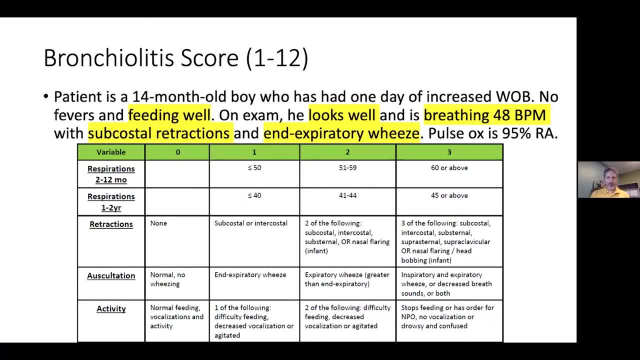 looked well breathing. 48, subcostal retractions and expiratory wheeze right. So we do this score, And so you can see zero, one, two, three, four, five. So he would get a five on this. 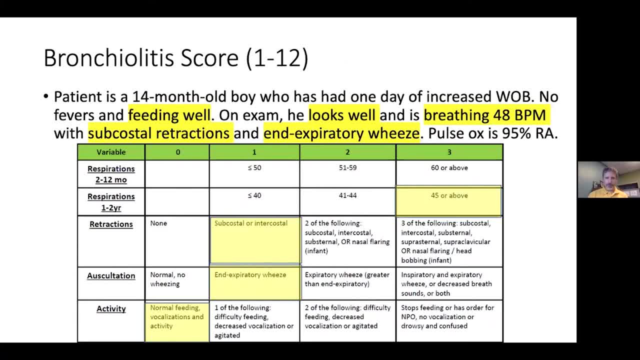 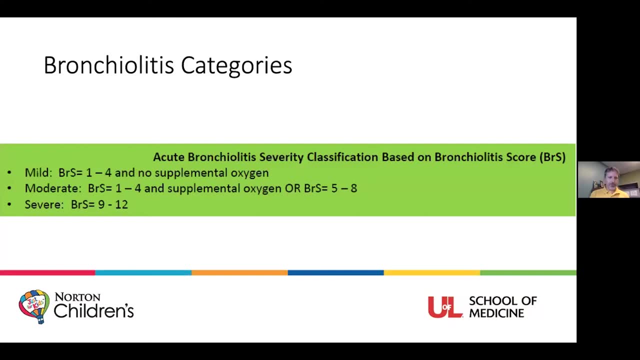 one to 12 bronchiolitis score. Does everybody see that? I hope Leave that up for a second. All right, So we categorize, categorize bronchiolitis based on that score we just did. So mild is they don't need any oxygen. 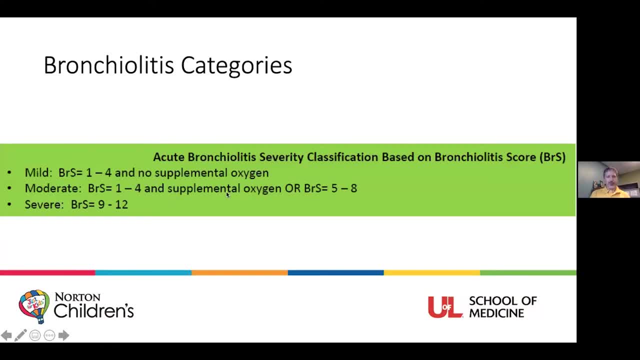 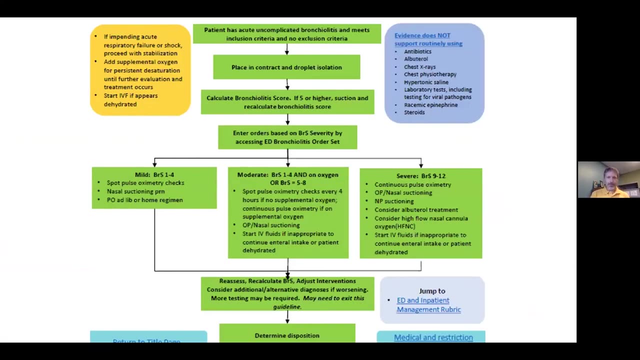 and scores one to four. Moderate is the scores one to four and they need oxygen, or the scores five to eight. that's off oxygen. And then, uh, severe is nine to 12.. Okay, And these categories help us to an extent decide what we need to do, And so here's this, um, part of this algorithm. 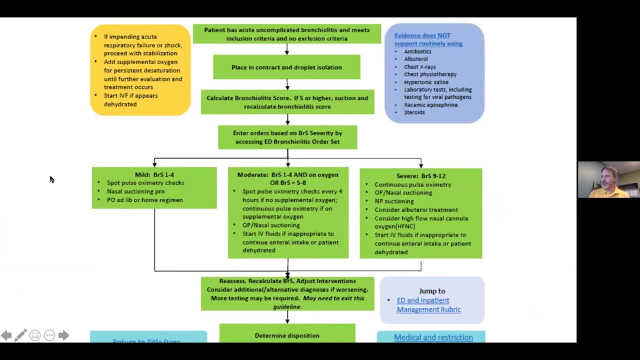 This one actually takes up several pages, I think, because of the complexity of the underlying and subjective. This one actually takes up several pages, I think, because of the complexity of the underlying condition. All right So, but basically, you know, and what would happen in this patient's? 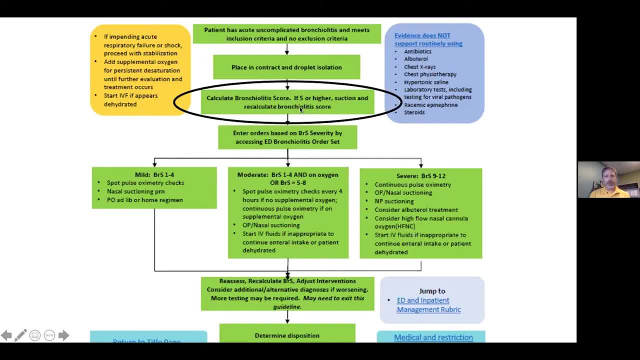 uh case, we calculate that score- It's five or higher, We suction and then we recalculate And there's sort of a lot of this: reassess, recalculate and adjust your interventions throughout this algorithm. Uh, you can see down here. it says again: excuse me, reassess. 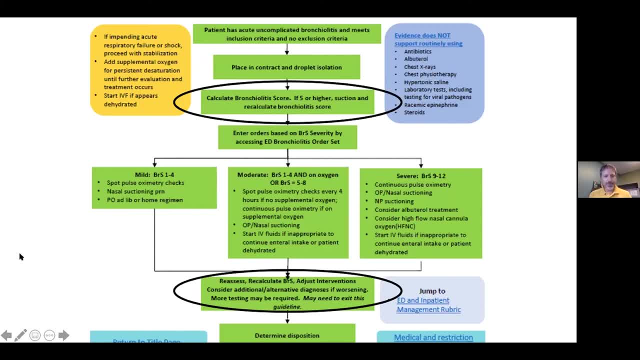 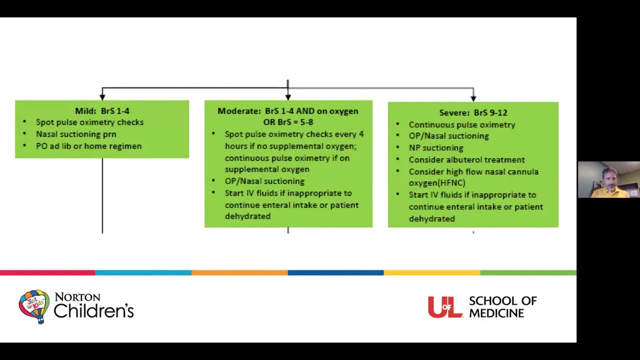 recalculate, adjust intervention, what I just said, All right, But this is sort of the first branch point, right? So after suctioning. so this is: you've calculated the score, you've suctioned them and you've recalculated. 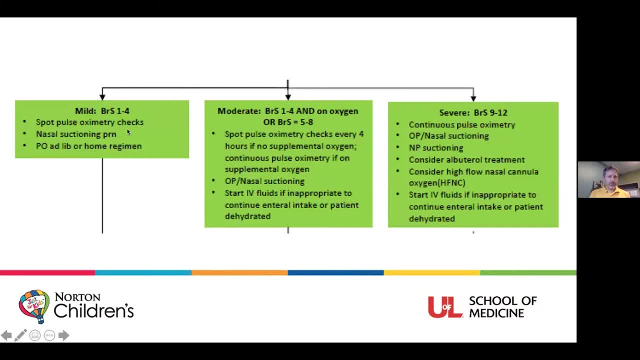 So if they're mild, you can watch. we watch all of these kids for a bit. Look at their pulse socks, suction them again if they need it, but you know, hopefully they're able to feed well, Uh and, and that's sort of the pathway to discharge. If they're moderate, uh, again we check their. oxygen. We do um more suctioning and we do fluid And and uh, if they're not able to tolerate PO and if they're severe, again same thing: pulse, socks, suctioning. consider albuterol treatment, consider high flow nasal cannula. 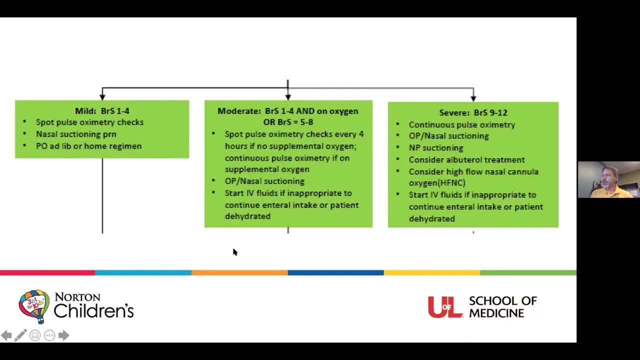 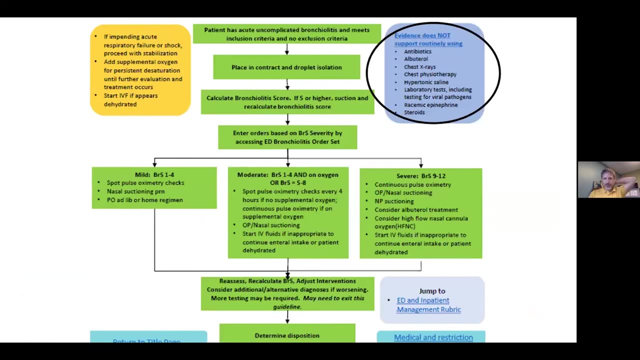 IV fluids if they're not able to stay hydrated or if we're worried about impending respiratory or airway failure. So consider albuterol treatment is interesting, um, because, uh, you know, up here in the corner this is on that main algorithm. It says evidence is not routinely. 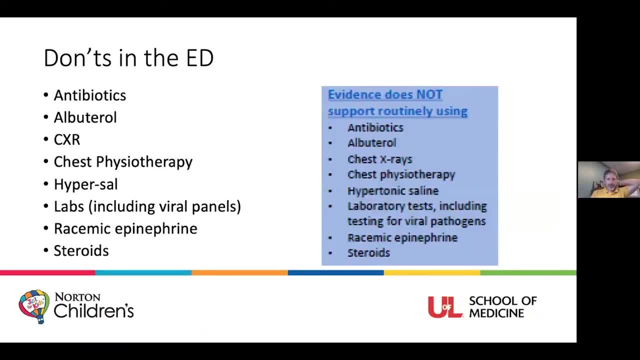 support, And then it lists these things. So if they're not able to tolerate PO and if they're going to make this big um, so it's essentially don'ts right. So if they have severe- what we call severe bronchiolitis, based on that score, we're supposed to continue albuterol. but we also say 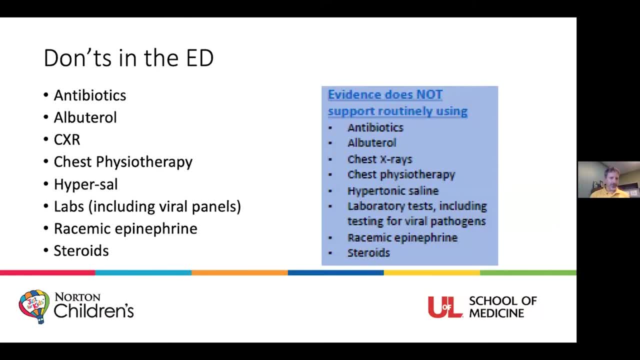 don't do albuterol And we also uh these other don'ts antibiotics, albuterol, chest, x-ray, chest physiotherapy, hyper uh, hypertonic saline, uh any sort of labs, or semicepinephrine or 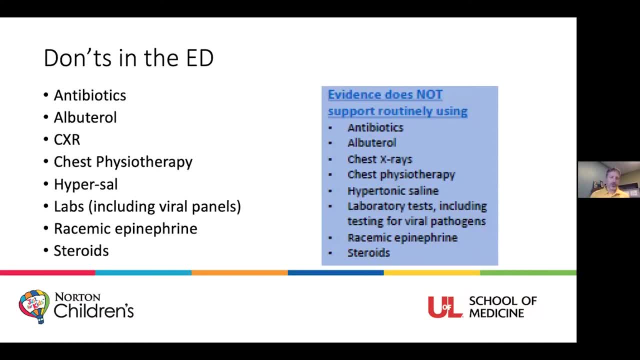 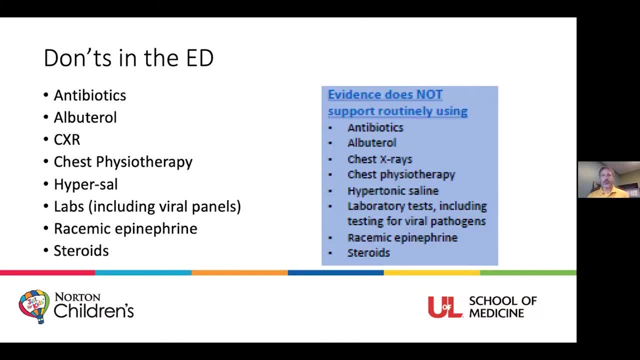 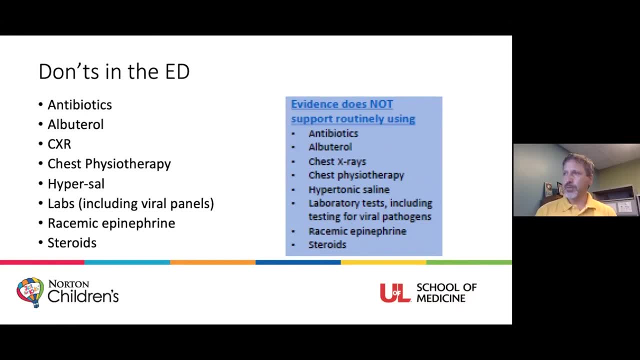 saline: 3%, 7%, 9%, uh, 6%, uh, you know that just periodically gets looked at from an emergency department perspective, None of it's been found to help very much at all. That's not to say that. 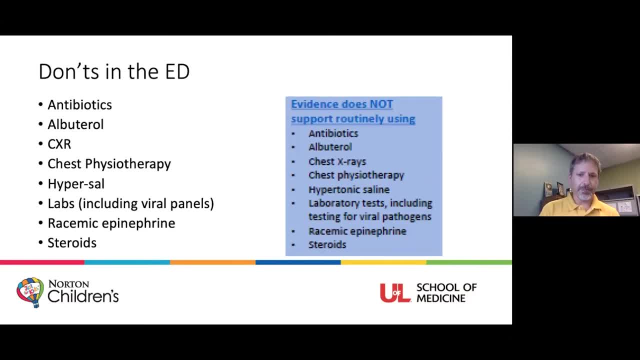 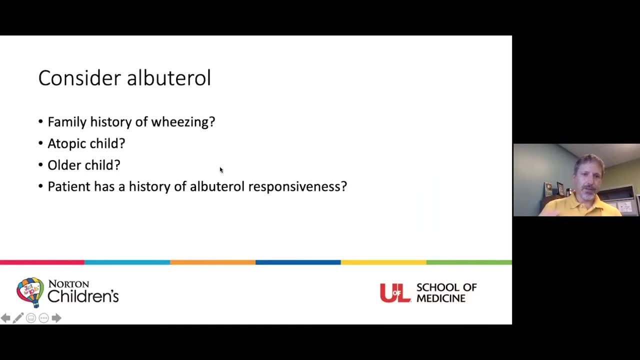 these aren't important parts of ongoing therapy. potentially, but really I wanted to focus on albuterol, because our own uh algorithms suggest that we consider albuterol, but it also says evidence does not uh support routinely using albuterol. All right, So when do we think about? 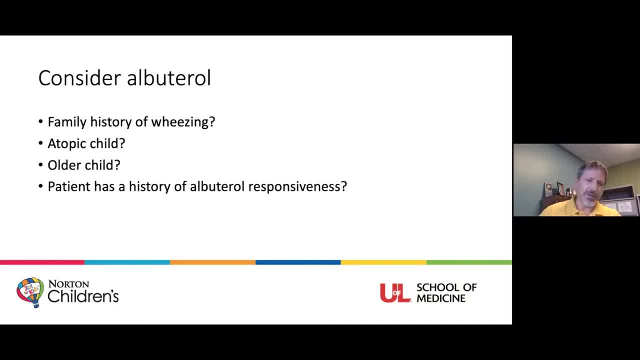 albuterol. Um, I think the the the times when I think about it at least, is when there's a family history of wheezing the child's an atopic child So has eczema. underlying is on the older end of. 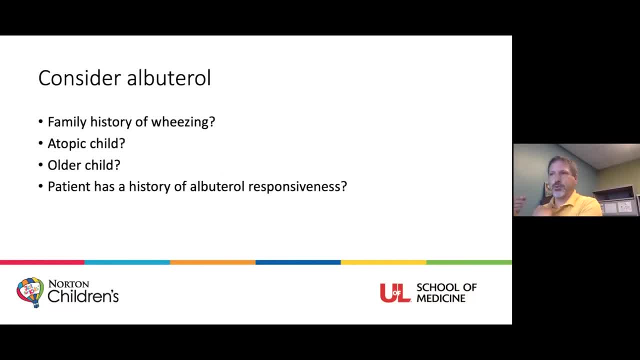 the spectrum, you know. so a three month old, I'm less likely to try it compared to a 22 month old who maybe has bronchiolitis and is really sick. Um, and you know. the other thing is if the family 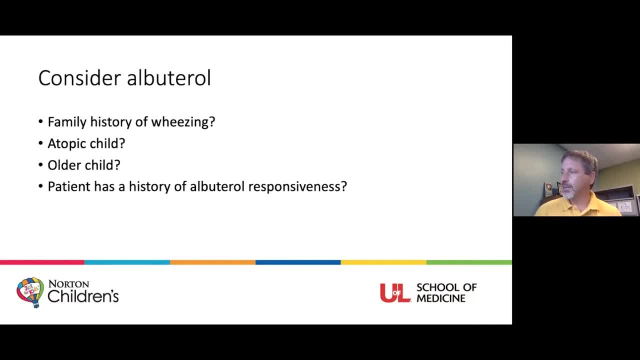 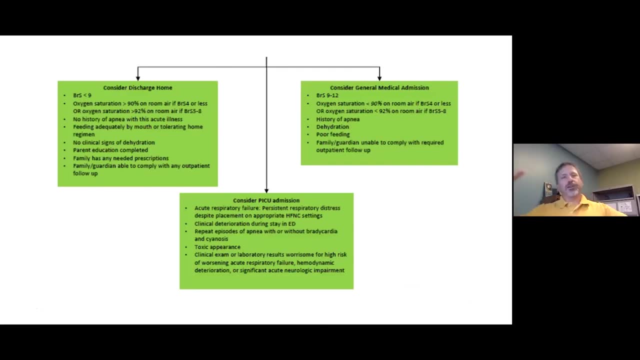 if there's something documented from prior visits, if the child's had respiratory illness before that's responded well to albuterol, then I suppose I would try it then. But in my opinion it's overdone and it's not usually very helpful. All right, So we've calculated the score. We've 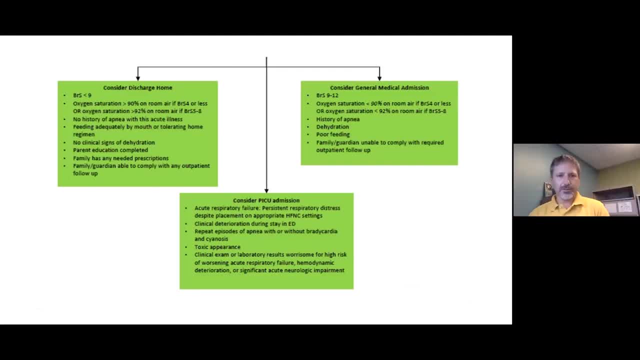 suction. we've intervened, we've reassessed, we've done all these things right. The child's been in the emergency department for a while now. So now, what do we do So we can discharge him home? The bronchiolitis? 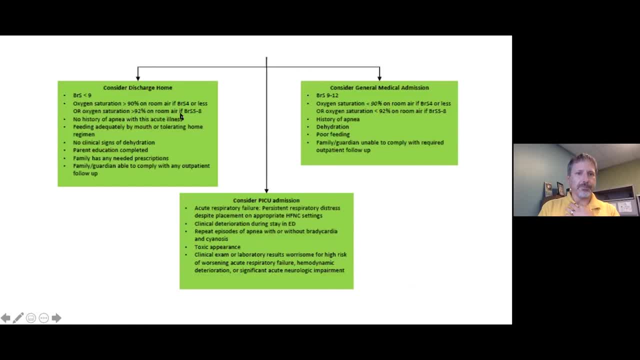 the score is up through eight, so less than nine. If their um blood oxygen level is okay, if they're not having apneas, uh, and if they're feeding adequately and not dehydrated, And um, you know, the the big one is, uh, that the fam, we're confident the family's going to show up for 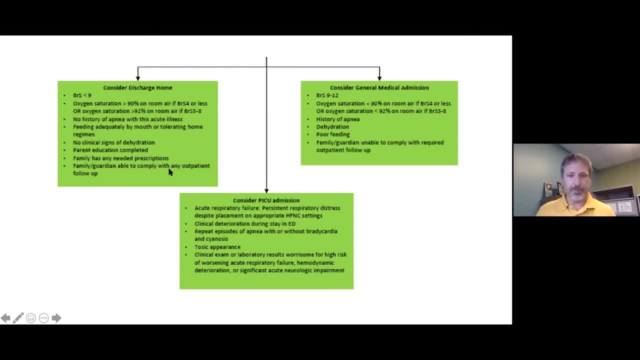 follow-up. We really do think that's important in all emergency department visits, particular in these. in these cases these children are higher risk, right, The score is nine to 12. after we do all these interventions And re-assessments. those are the kids we think about bringing in along along with, obviously. 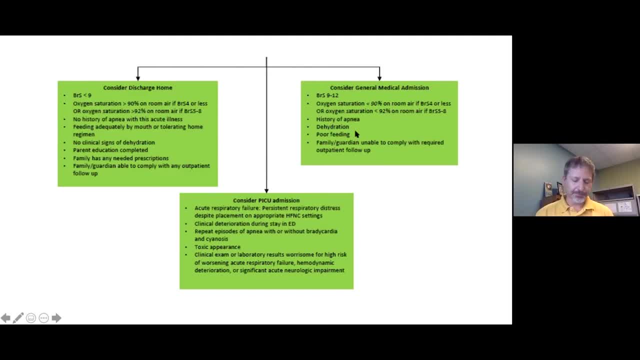 hypoxia, if they have a history of apnea, dehydration, poor feeding or, frankly, if we think family's not going to follow up. And then some of these kids wind up in the uh, in the PICU, Uh. 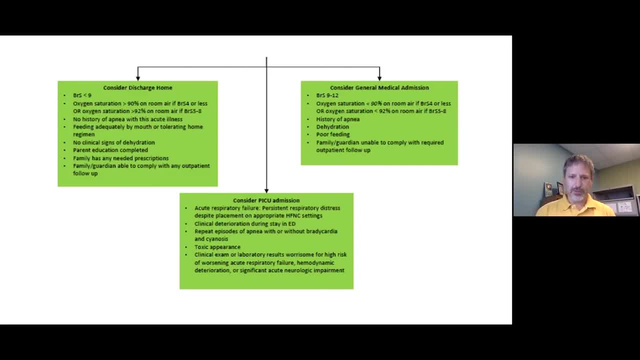 so these are the ones that have persistent respiratory distress, despite uh um appropriate oxygen or high flow nasal cannula. Um they deteriorate while they're in the ED. We observe them having apneas. They look toxic Um you know these sorts of things that are obvious sort of for the ICU um those patients. 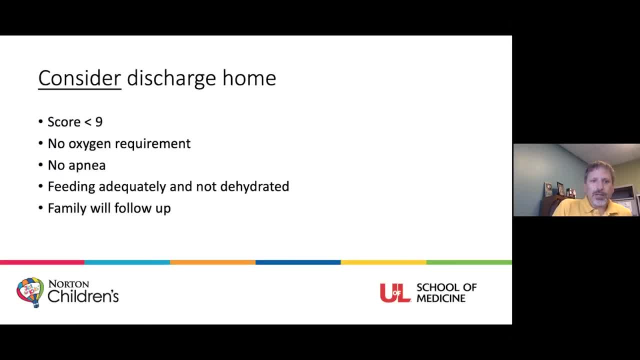 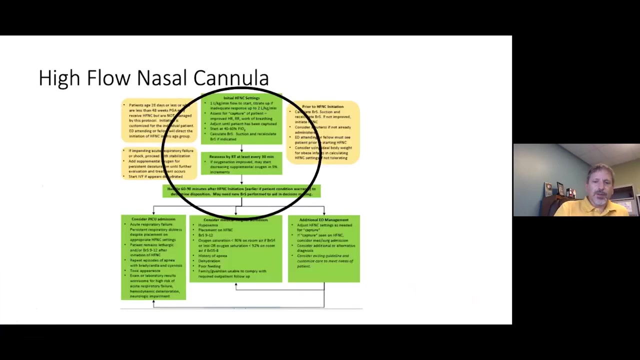 go to the ICU. So again, consider, consider discharge home. Those are the criteria. Consider admitting to the floor with those criteria and then consider PICU admission, All right, So I wanted to talk a little bit about high flow nasal cannula in this setting, Um, and I'm going to 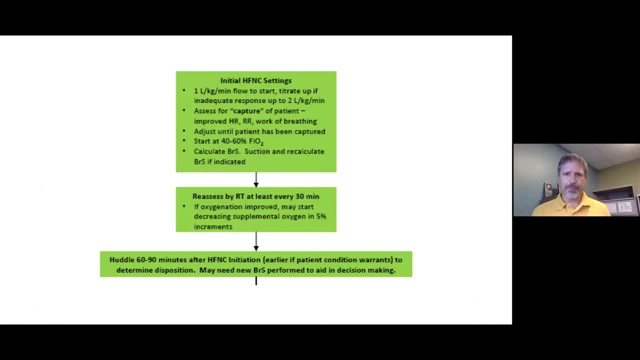 make this bigger. Yes, Right, So we start um at uh one, uh liter per kilogram per minute of flow and we'll titrate that up to two liters per kilogram per minute of flow to try to make the. patient better Once we get past two per kilo. those children all need to go to the ICU. So the sort of limit of tolerance for taking care of these patients on the general floor is two uh liters per kilogram of flow. 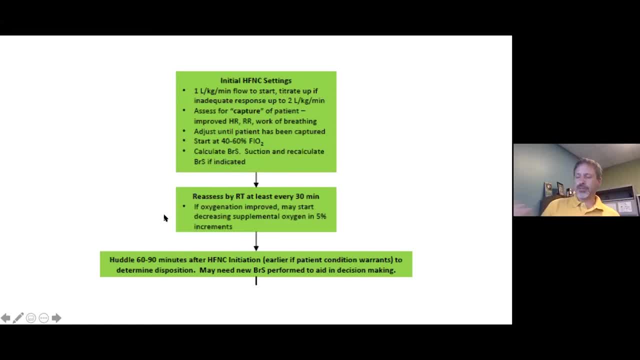 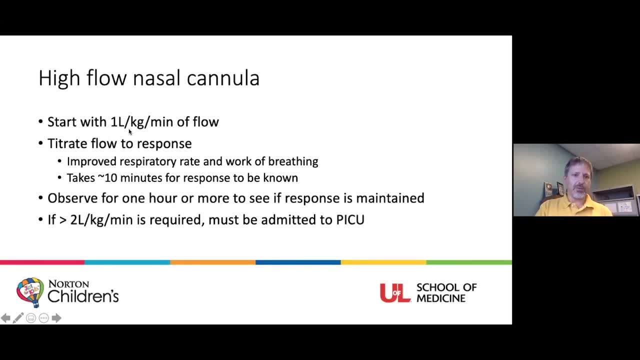 All right, But we can't just put them on it. You kind of have to leave them on there for a bit and then reassess them frequently and decide how well it's working All right. So again, we start with uh one liter per kilogram per minute of flow, and we titrate flow to response. 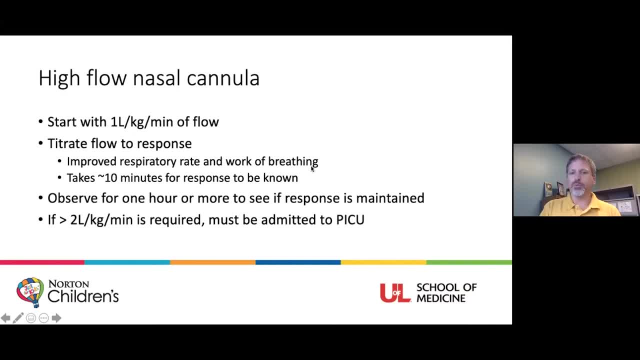 Uh, and response in this case means the respiratory rates coming down. work of breathing is improving to a lesser extent. The pulse oximetry is doing better, although it it only really helps with that at higher levels of FiO2.. The other thing with high flow nasal cannula is: it's not you put. 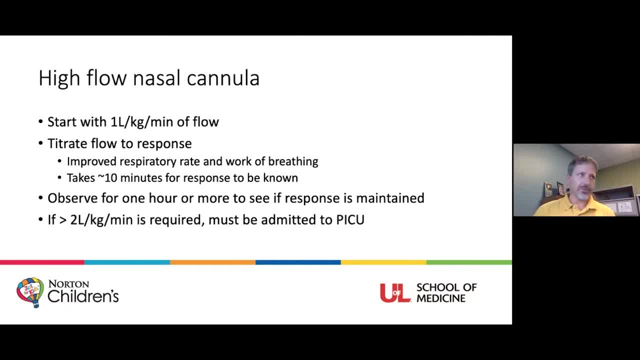 it on and they immediately get better. It takes 10 or 15 minutes for the child's physiology to adjust to the flow, essentially for us to know if it's helped. So we do all that. Then we observe them uh and see if they're uh able to maintain their response on whatever flow we have them on. 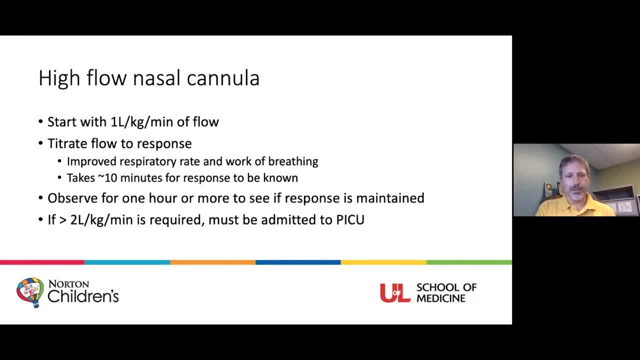 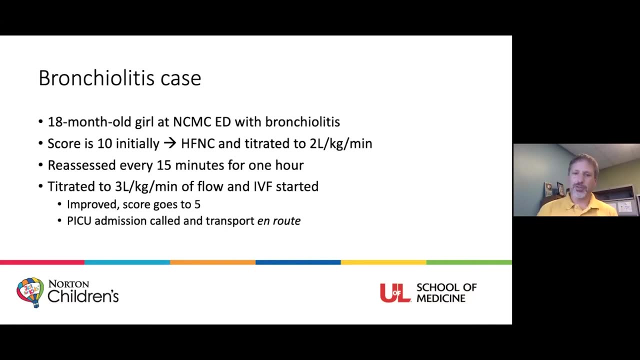 Uh, and then again, some of these kids, if they get up more than two liters per minute, uh, per kilogram per minute, we wind up admitting them to the PICU. All right, And so just to help you understand a little bit about the how difficult this is to care for. this is a case I had two or three years ago- two years ago I don't remember. it was pre-pandemic. So I was at NCMC, Northern Children's Medical Center out in Brownsboro by Costco. there I had an 18 month old girl. she had bronchiolitis. Nice family kid looked okay. I. scored her a 10. initially. She was a little bit older than me. She was a little bit older than me, Um uh, because of her work of breathing and her respiratory rate. mom was actually an anesthesiologist. We talked through. everything started on high flow. nasal cannula titrated her. 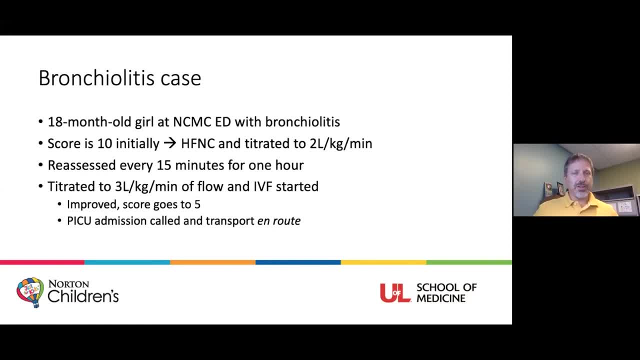 up Our practice at NCMC. that's a. it's a 16 bed ER. You're kind of right there in the middle of things. I reassessed her frequently. It wasn't terribly busy that afternoon. I remember evening. 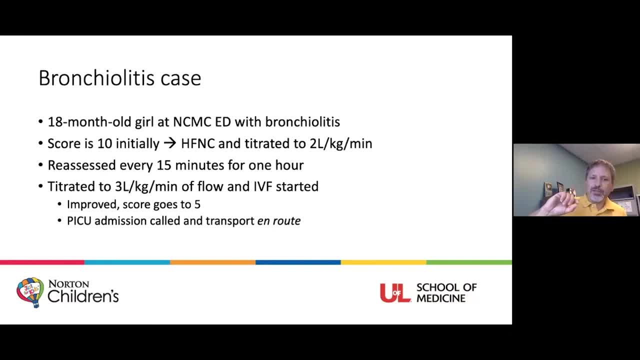 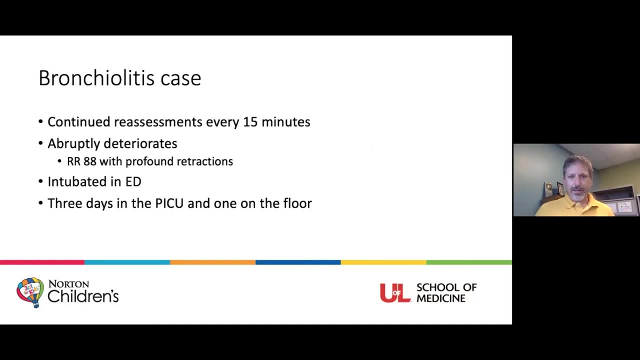 whatever it was. Uh, but at any rate I eventually had to titrate her further, up to three liters per flow And she improved. her bronchiolitis score went down to five. I called the PICU and we called for JFK transport and they were on their way there. Uh, and I continued to reassess her. cause it still. 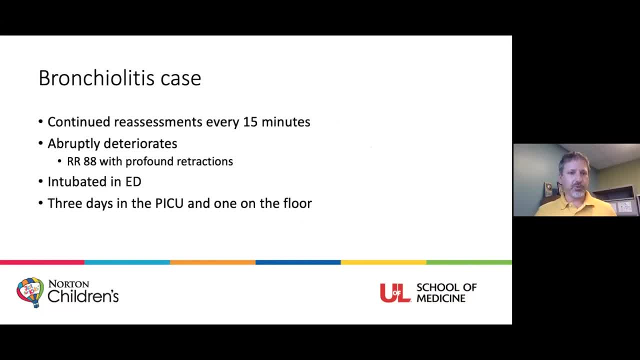 wasn't busy. And then she abruptly deteriorated out of nowhere. Her respiratory rate went up to 88. She was retracting everywhere And I intubated her and she wound up in the PICU for three days and then went to the floor and eventually went home. So the story had a happy ending. The point: 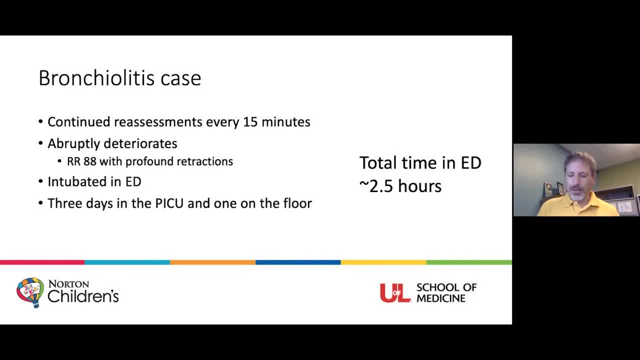 is. this child was only in emergency department for two and a half hours total And they went. they went from sort of looking okay-ish to getting intubated Bronchiolitis, just it's. it's a very challenging disease to nail down. Some of these kids get abruptly worse and it's just hard for 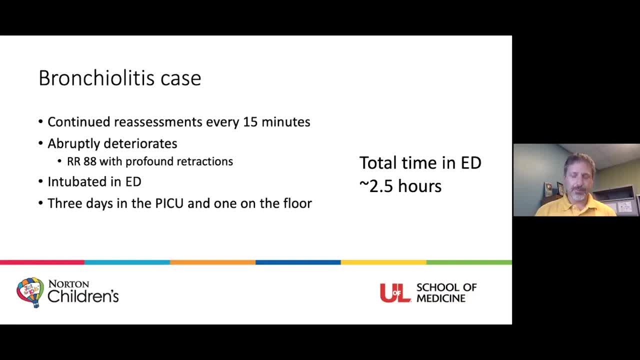 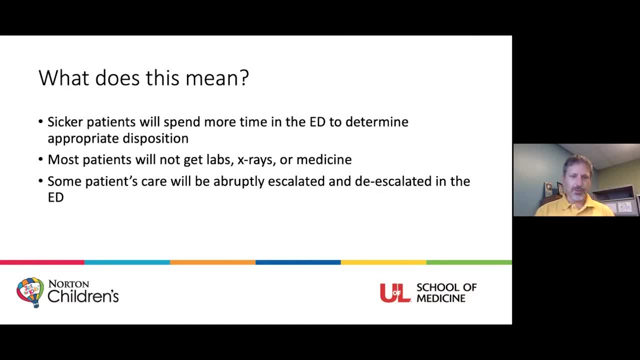 us to know which ones it is going to be. So what does all this mean? Um, sicker patients spend more time in the ED to determine the appropriate disposition, like we just talked about. Most patients will not get labs, They don't get x-rays or any kind of medicine, And then some patients again- uh, their care will be. 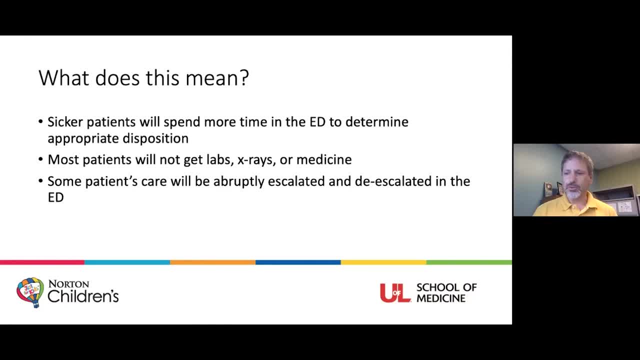 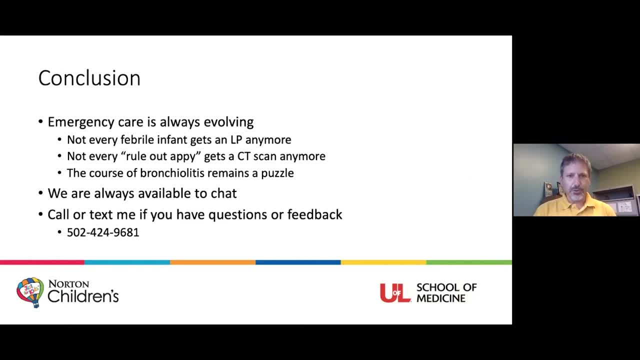 abruptly escalated and deescalated in the emergency department, as we just discussed. All right, So in conclusion, emergency care is always evolving. Remember, not every febrile infant's going to get an LP, not every rule out app. he gets a CT and bronchiolitis is can be. 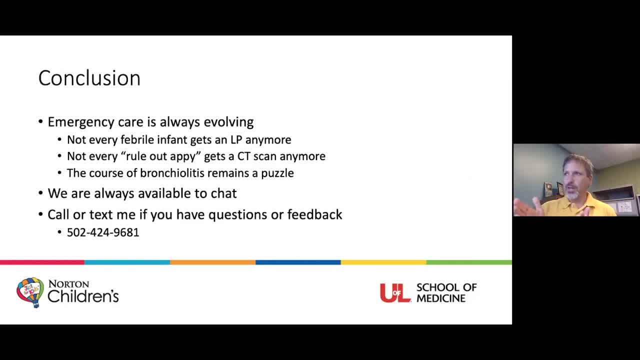 puzzling to to care for. Also, remember that we're available in our emergency departments 24 seven. You can call us in the chat box. We'll be right back. Uh, I'm really excited to cover the, the chiropractic. I'm excited for this, So, uh, 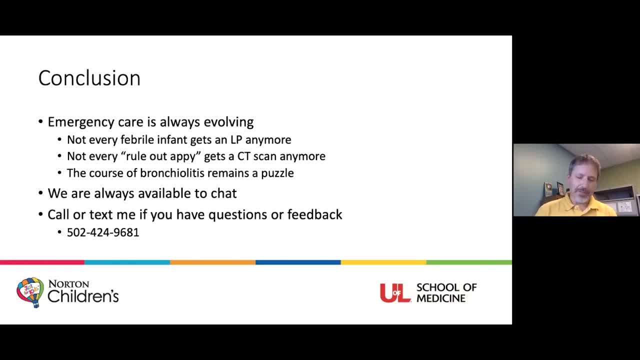 what we, uh we're going to talk about today is- uh is patient safety and child care, And again we're going to talk a little bit more in-depth about how that works and how our patients, our pediatricians, are going to get some help to do that. But what we're 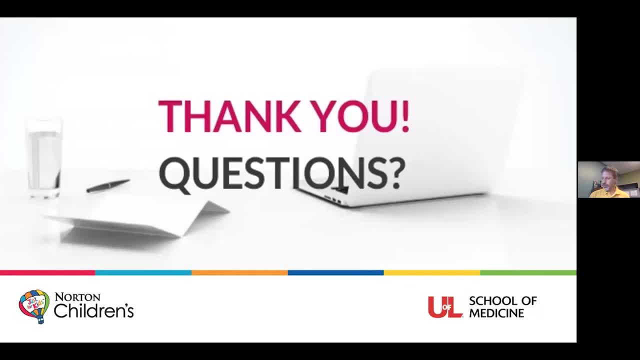 going to do is we're going to talk a little bit about what we do for them And then we'll get them in the department And you can get a doctor to talk to you- one of our fellowship trained PEM providers- And then again there's my number. again, please call or text me text. 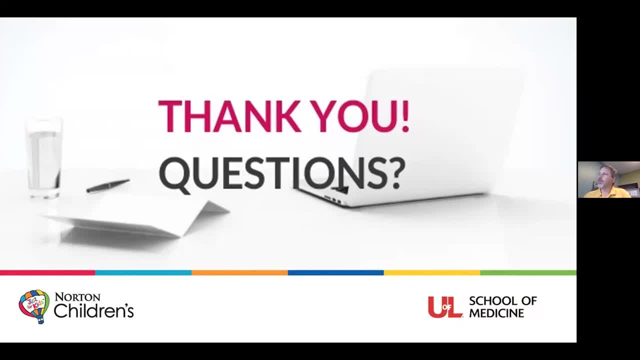 me now to introduce yourself. Uh, I'd love to hear from you if you have any questions or feedback. Thank you all for your attention. Are there any questions on this talk? low temperature and the current recommendations for what temperature warrants further evaluation. I can. So we're actually looking at our experience here over the last couple of years with the so-called hypothermic baby, And there's some data coming out around the country again- emergency department data. Other people are looking at this as well. So for most of us we look at 96.5 Fahrenheit or 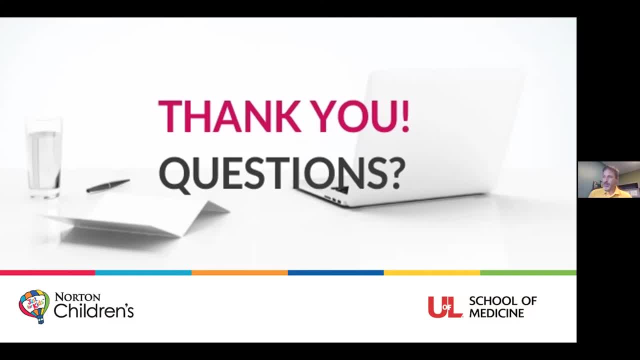 lower as hypothermia, And the reality is we're still combing through the data, but it appears that we do a lot of testing on these children and they're all fine. The ones who aren't fine are not the two-day-old or three-day-old who's 96.2 in your office. They probably have a reason. to be hypothermic because they're little babies. It's the three-week-old who's hypothermic, or the two-month-old that's hypothermic. Those are the kids that wind up having serious pathology because they really don't have a good reason. 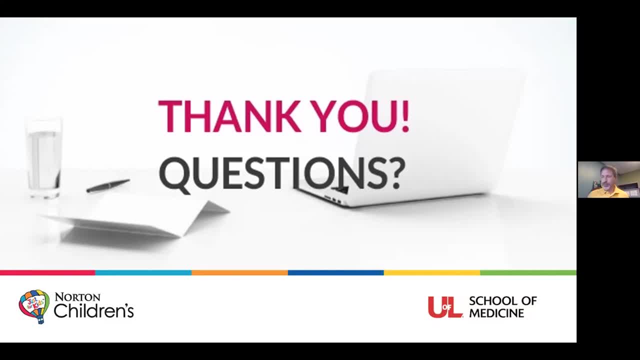 But for the most part these children in the first several days of life they get hypothermic. they're all fine And we're going. there will be, I suspect in the next year or two, further guidelines coming out about how we should evaluate those children. 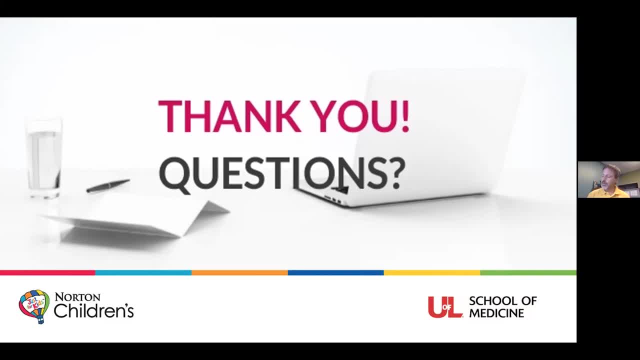 Okay, Next question: Can you comment on why rhino enterovirus is listed specifically in the physician discretion section, which seems to be an exclusion for home care being, And it's in the In the febrile 29 to 60-day-old part? 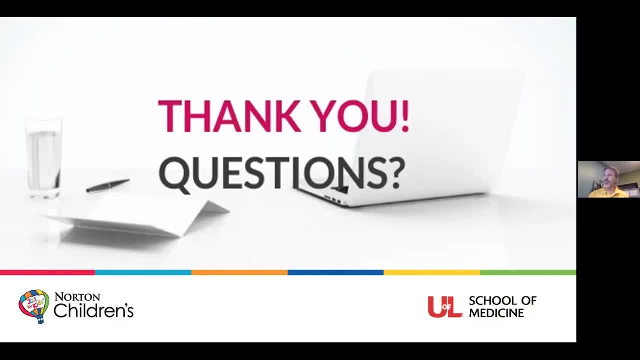 Yeah, Yes, That is because it is the thing that is most frequently positive And we actually see plenty of positives in children who don't have fever. And so I think most of us are not willing to, and as a group we sort of decided we're not willing to chalk up the fever to rhino enterovirus. 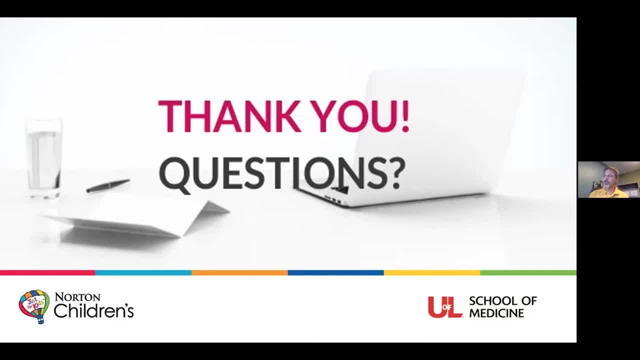 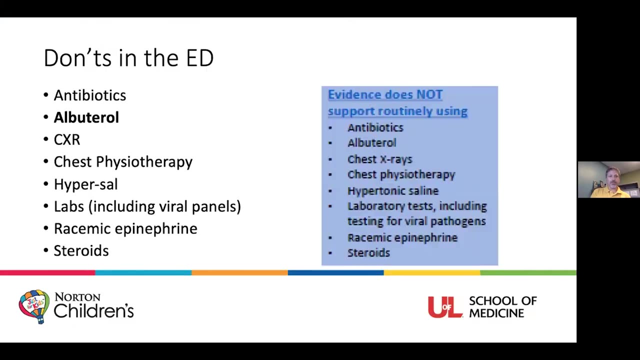 infection. All right. Next question: Comment on the don'ts That you listed. So if you don't use albuterol, do you use any respiratory treatment And if so, what do you use? I'm going to go back to don'ts. There we go. No, we don't use any respiratory treatment. That's. 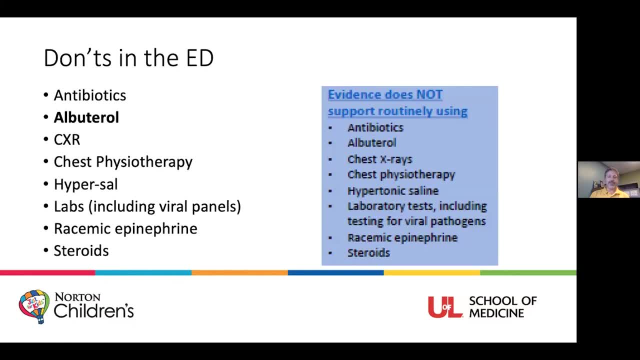 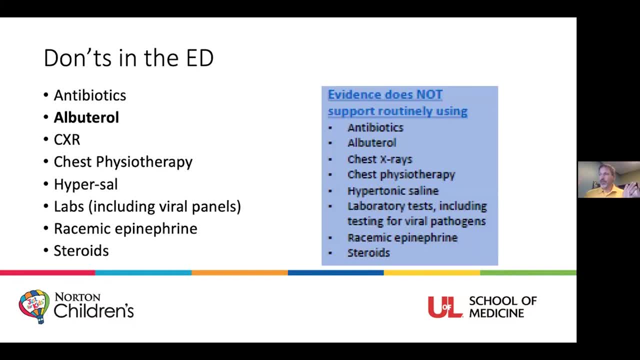 It's different in the intensive care setting or the general medicine admitted setting, But in the emergency department setting these things don't affect any meaningful outcomes, which for us is deterioration of disease, need for admission, need for ICU ability to discharge those kinds. 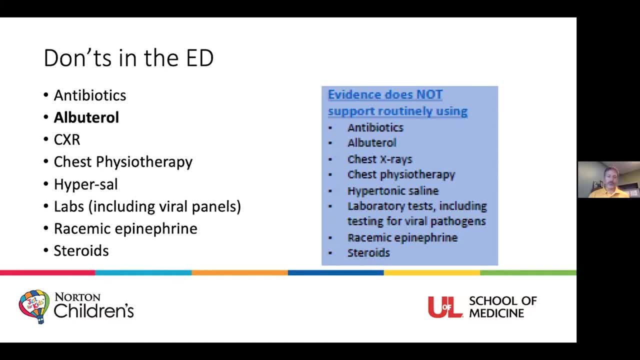 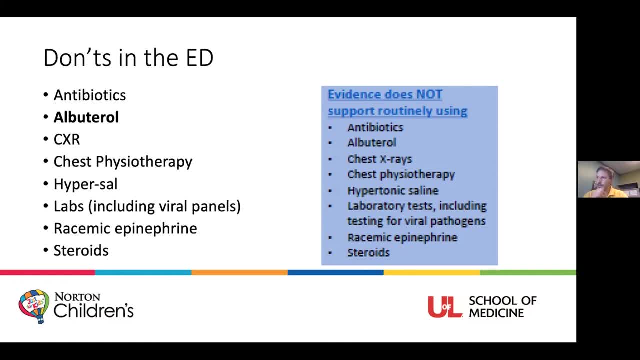 big thing And I think it's a big thing And I think it's a big thing And I think it's a big thing where we see it effective. Next question: are you doing an appendicitis study with antibiotics only and no surgery? 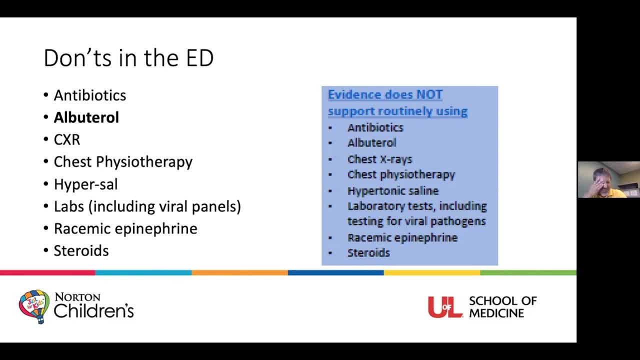 Yeah, so that's been looked at. That study is, I don't believe, any longer active. I don't know that they ever wrote up the, so we participated. it was really the surgeons that drove this, but they participated in a. it was a national multicenter study And I don't know that I've seen it. 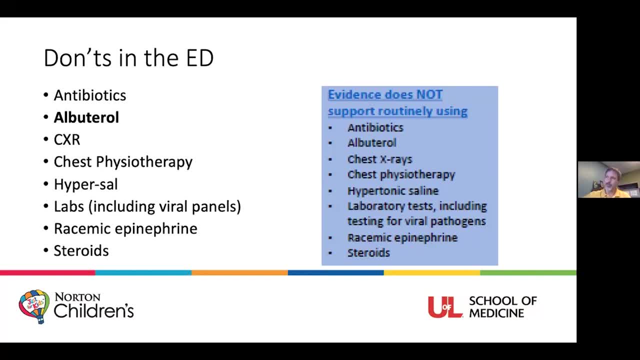 published yet To see what the final outcome was, But yeah, we're just seeing the results of that. That is something that was ongoing for several years. Okay, Are the algorithms available to share Or are they proprietary? They are available on insight, And so those of you who are part of Norton Children's Medical Group. 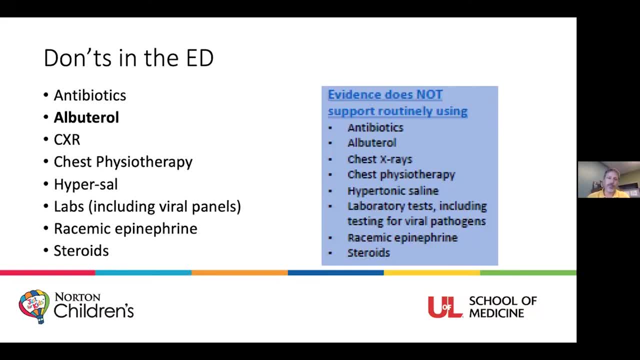 they're certainly available, for They're not proprietary. I mean, if you send me a text or something, I'll figure out how to email it to you or text it to you or whatever. That's fine. Okay, no urine testing in the appendicitis algorithm. so do you check urine in that, in those patients? 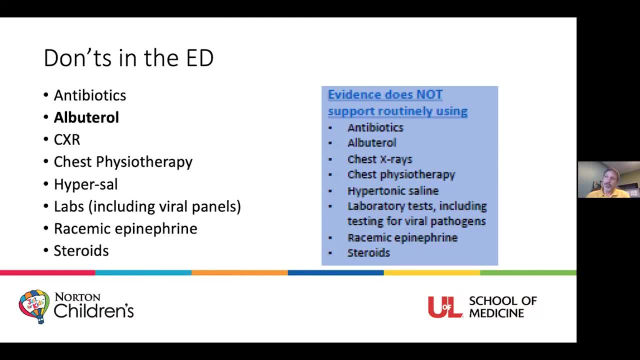 yeah, absolutely, um the uh, you know it's just not part of the evaluation for appendicitis. it used to be, because you used to think about it in terms of: um, some, especially girls, would get sterile pyuria with appendicitis. but now we're checking, so, in girls, make sure that they're not pregnant. 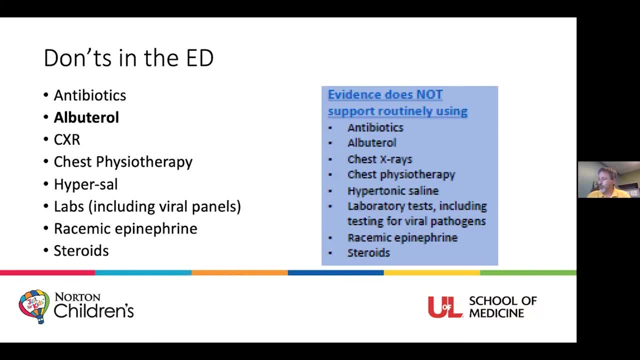 because we don't want to miss an ectopic. and then, um, you know, to look for possible uti, but we're not really looking for appendicitis. in that case we do check your, their urines, as the answer your question, and then are there any new pathways under development? so the big one, that's, that's. 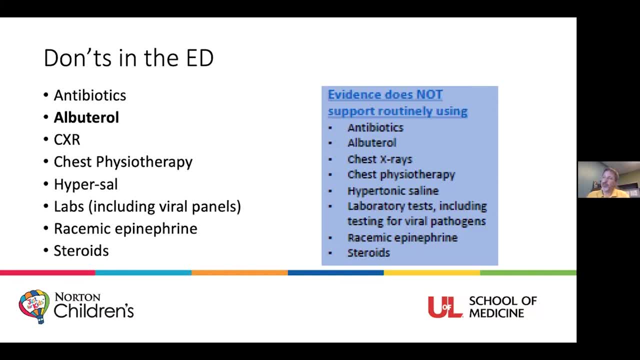 going to be coming up next is to more formalize how we treat asthma in the emergency department and really fold that into the inpatient asthma pathway, so sort of utilizing the same. it'll be a similar structure to the bronchiolitis pathway, i think a little more.